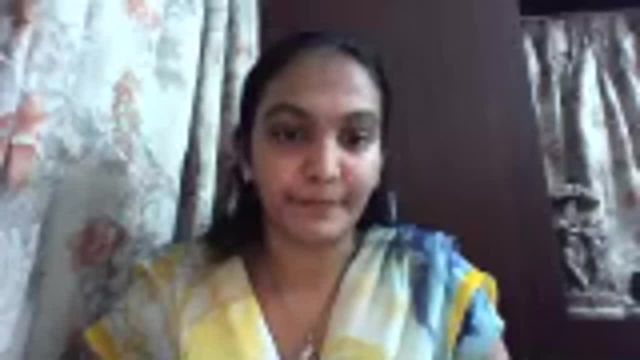 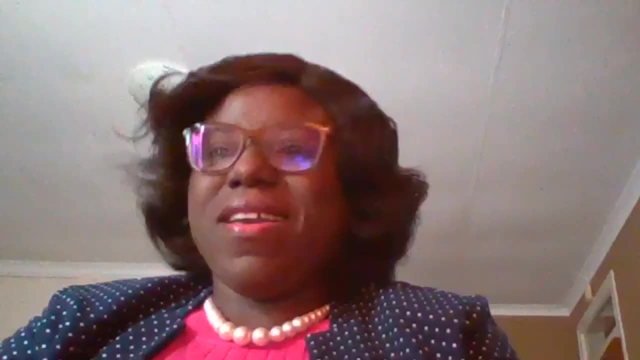 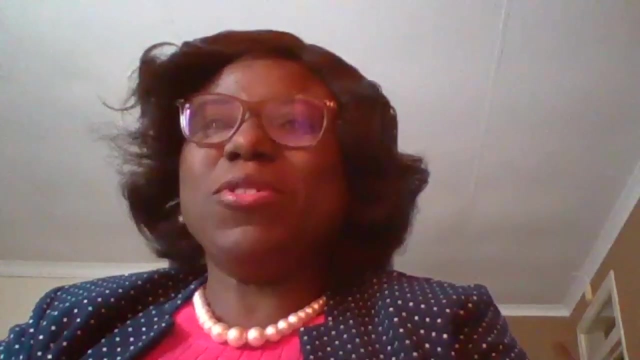 She is a member of prestigious South Afterlife Research Association, African and Academy of Science and Register. Welcome you, ma'am. Welcome you, ma'am. Thank you, Dr Taya. Good day to everyone And for me, from Johannesburg, I will say good morning. 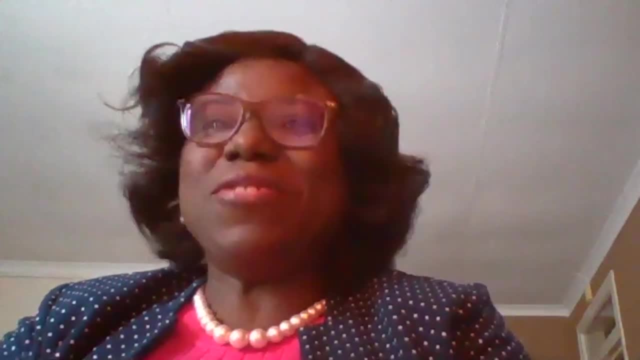 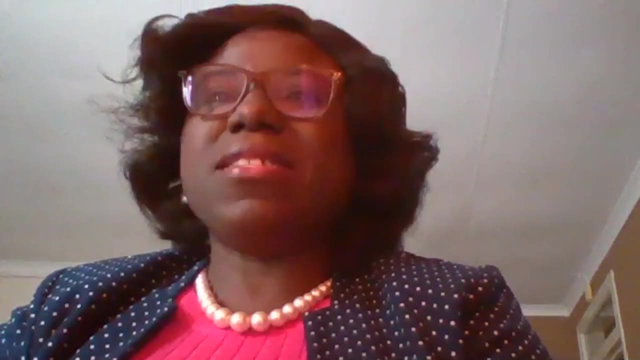 This is about half past 10.. In India it is good afternoon because you are at 2 pm already. Thank you very much to Dr Taya, And I would like to start to also seize this opportunity to thank Prof Swadesh Singh. 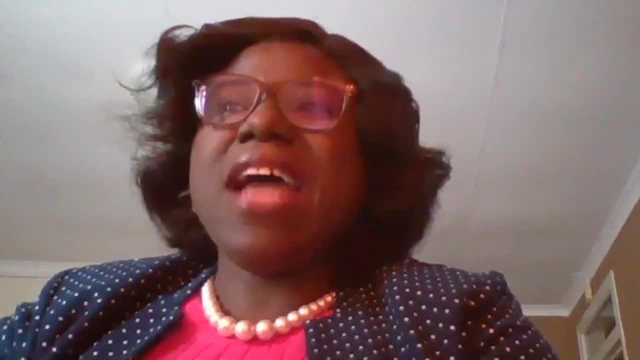 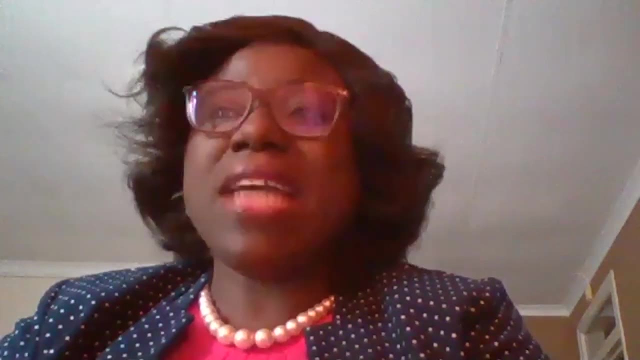 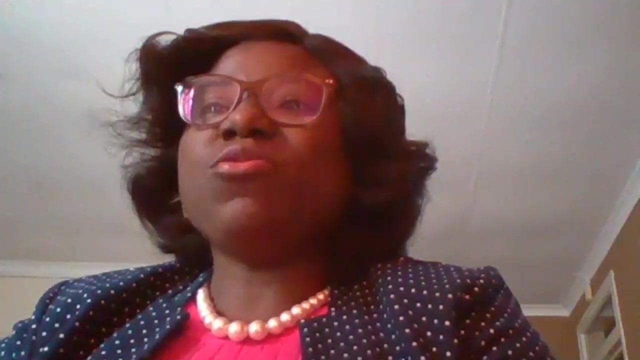 who has been my collaborator for a number of years and who is the person that contacted me, and he's the one, the brain behind this program, And thank you very much to Prof Singh, And to other committee members as well, to be able to put this. 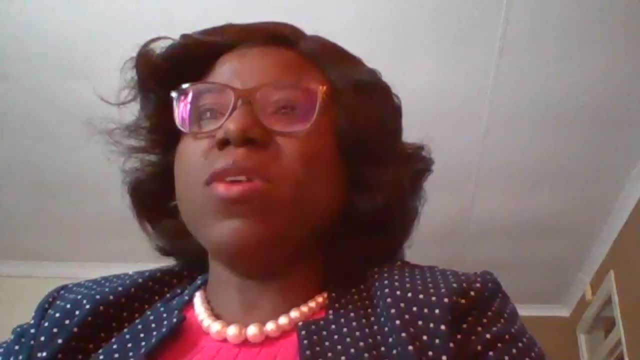 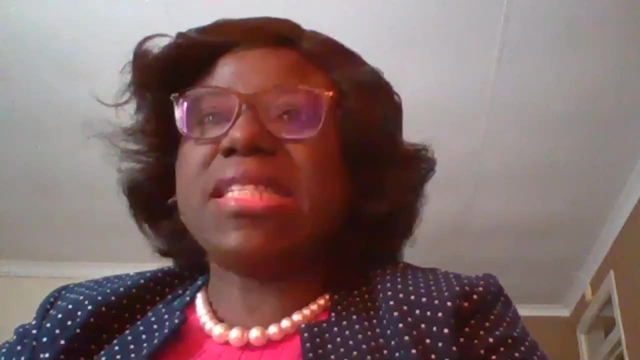 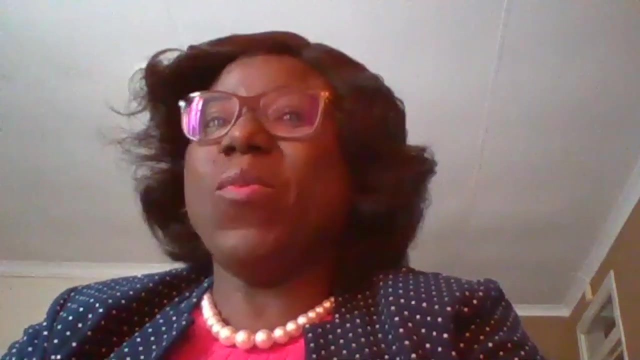 the online development program together. I want to start by commending your efforts to be able to achieve this feat. Looking at my screen from here, I see 411 participants. This is a huge number and I'm really wondering how you were able to pull such a number together. 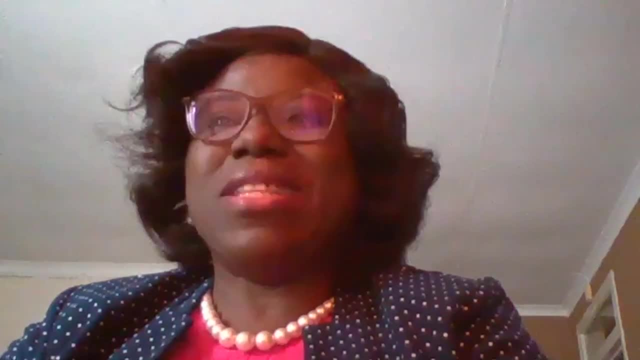 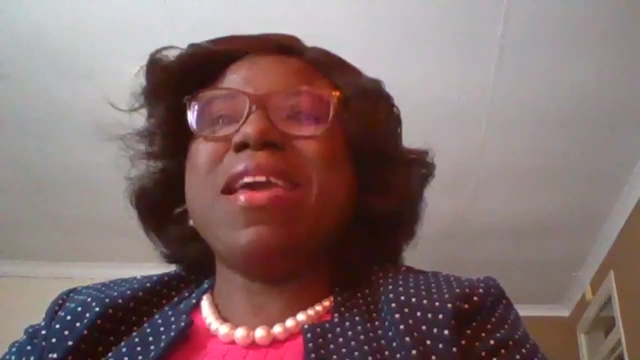 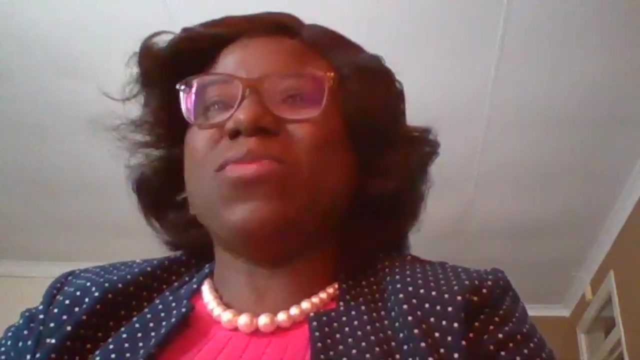 amidst the lockdown and everyone facing one or the other. However, the COVID-19 pandemic has really enabled us to learn and unlearn, and we are really taking challenges. We are pulling on and moving forward, irrespective of the pandemic across the globe. 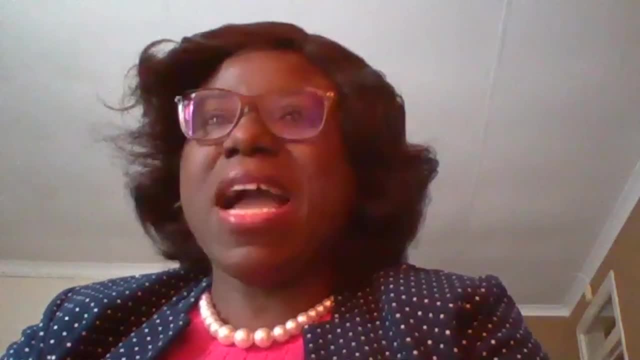 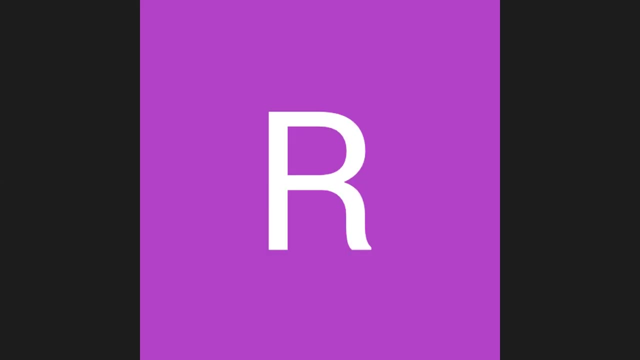 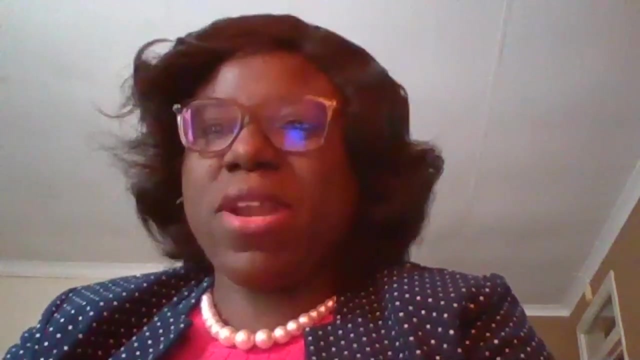 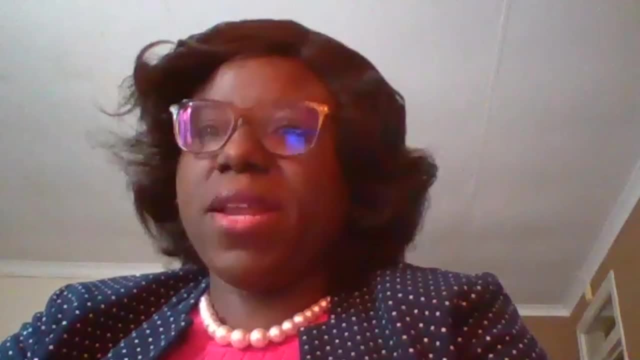 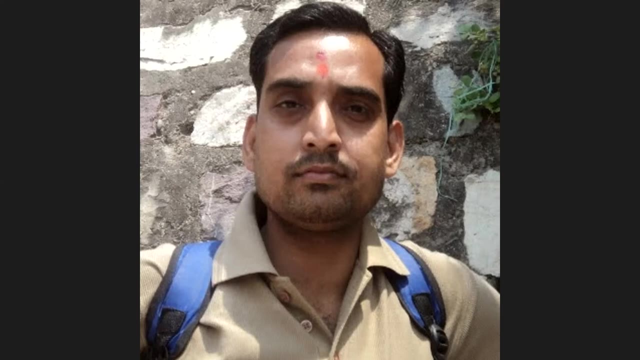 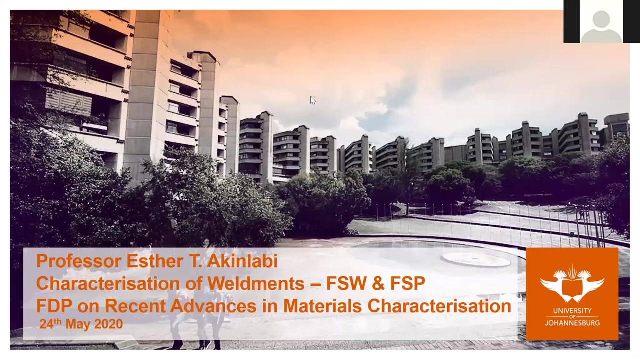 I will now move ahead to share my screen. All right, so I'm now sharing my screen and the topic before me is a characterization of weldments and, in particular, from my research experience in the field of friction stir welding and friction stir processing. 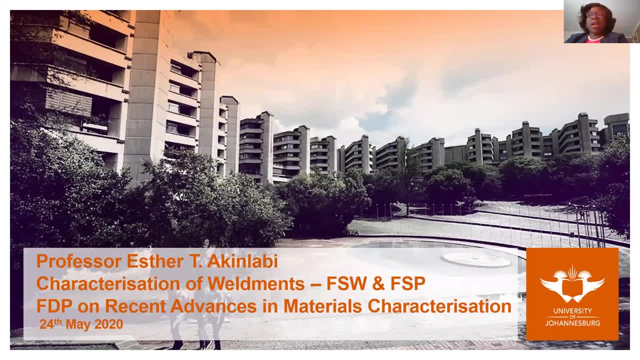 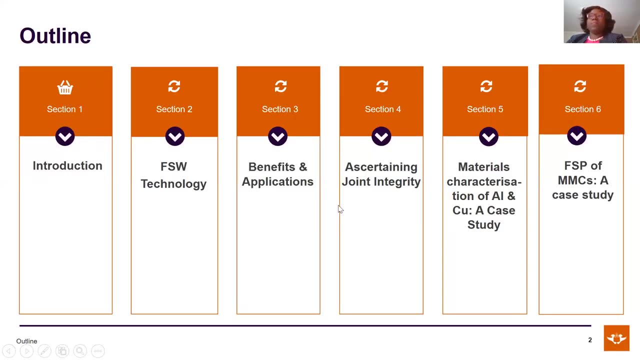 This is an FDP program with the theme Recent Advances in Materials Characterizations. This is the outline of my presentation. I will start with the introduction into the field of welding generally, Then I will narrow into the friction stir welding technology. I will share with you some benefits and applications. 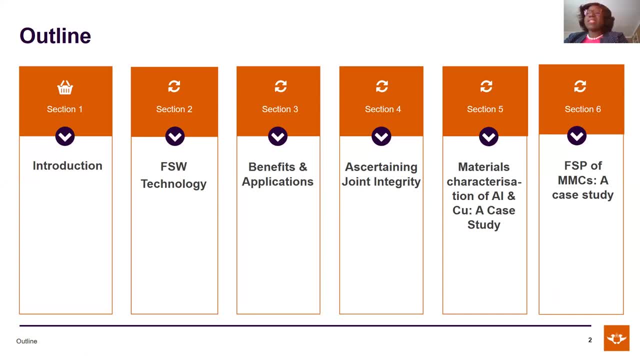 From there I will move on to highlight how we can ascertain joint integrities, particularly in the field of friction stir welding. I will then present some materials characterizations, with a case study of aluminum and copper, the similar welds, and, lastly, I will share some work that my team and I have done in 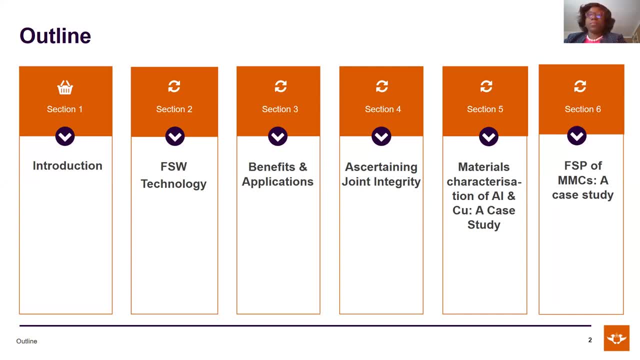 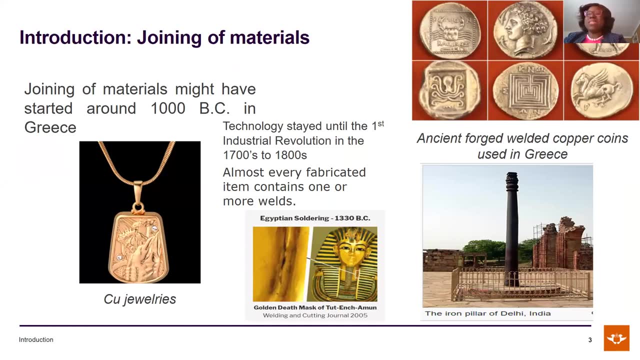 the field of friction, stir processing, Joining of materials is believed to have started around 1000 BC in Greece, and they started by having to produce jewelries. Greece's jewelries are known to be very famous, ancient and many people still value them. 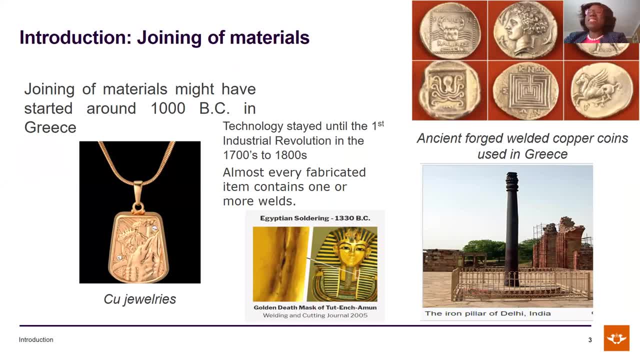 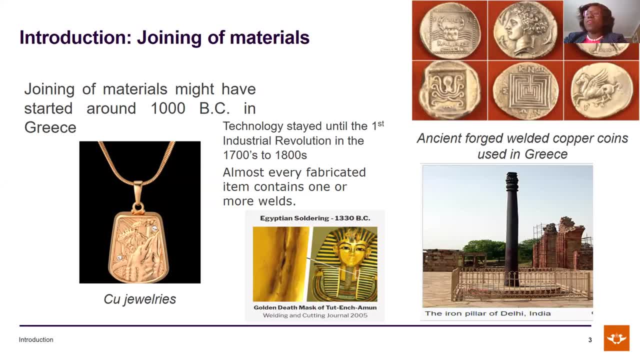 But for India. when I checked the history of how far, of how long, welding had been used in India dates back to so many years as well, thousands of years ago, and I came across a particular interesting the iron pillar of Delhi in India that this was built by. 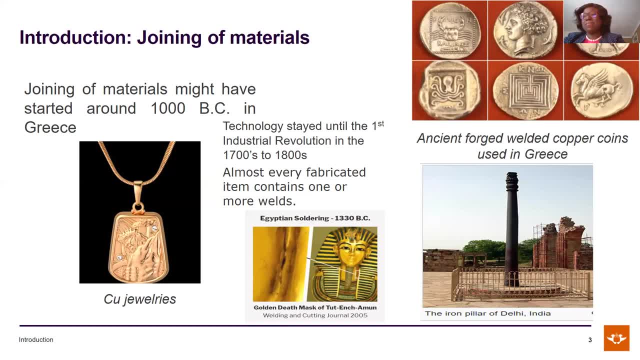 using the welding technology in 310 AD On the African continent, I saw the Egyptian soldiering of the golden death mask. That was a well used. the welding technology was used in 1330 BC. However, welding technology remained primitive Until the advent of the first Industrial Revolution in the 1700 to 1800. 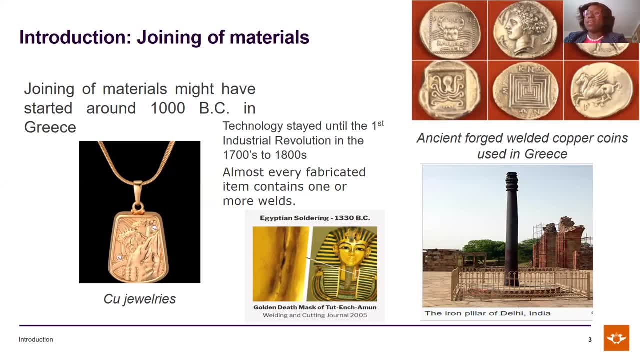 And you will agree with me that almost every fabricator item that you can think about at home, in the office, in industries and all over the world will always contain one form of joining, and welding technology has been in the forefront of the ability of manufacturers to be able to. 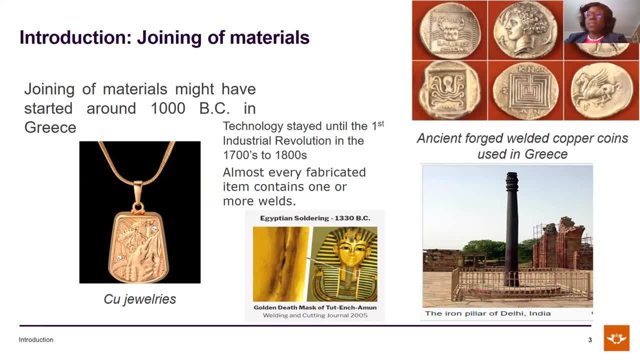 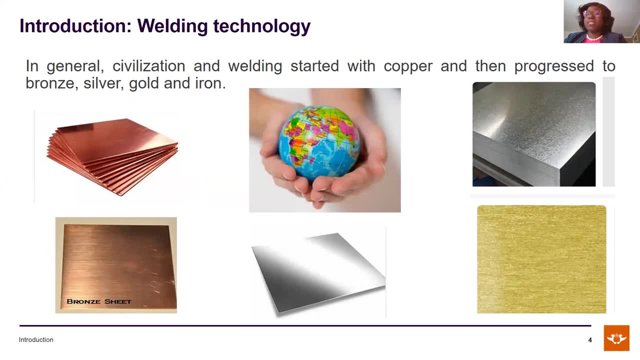 join two materials together. With this background in general, civilization and welding started with copper and then progressed to bronze, silver, gold and iron across the manufacturing industries, But then, over the years, with the advent of the second industrial revolution, the third 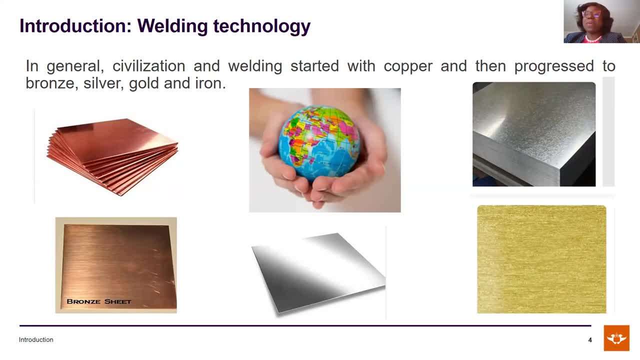 the fourth and even the fifth industrial revolution, currently in Japan. we then realized that welding technology has now been used in joining metals, plastics, composites and so many materials globally. Hence the importance of welding technology and, more so, the importance of researchers. 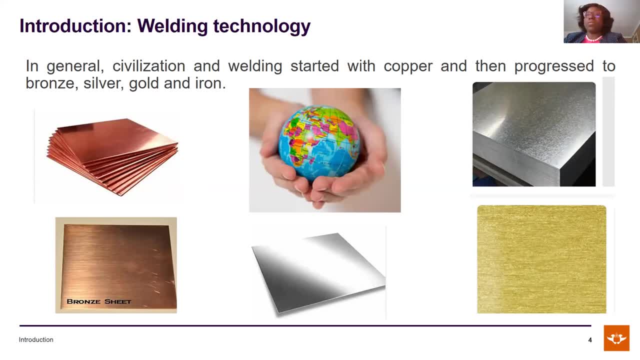 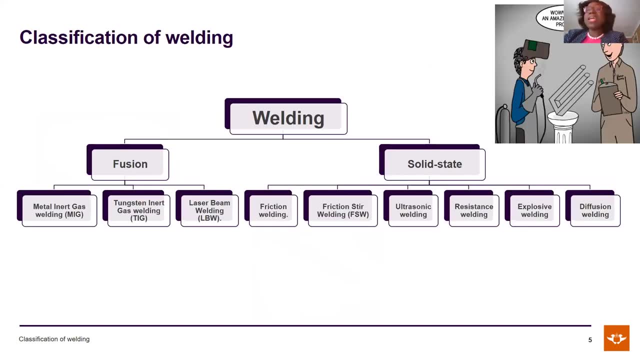 knowing fully how to characterize the welds to be able to ascertain the joint integrity. With this background, still on background, transmission of welding. I'm not sure how many of us participants are very familiar with this particular field. I'll put this slide here but I will try not to bore you. Having 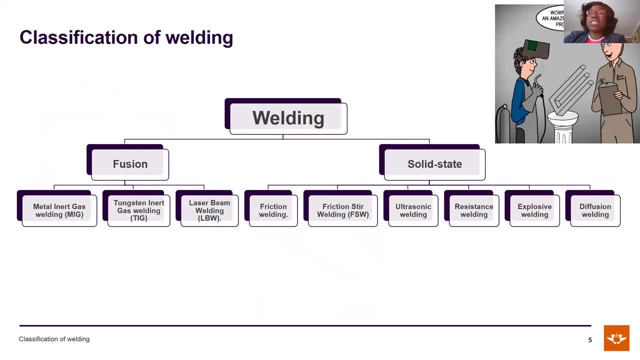 the general classification of welding into fusion welding technology, which is the conventional welding technologies and the solid-state welding technologies. Under the fusion welding, we have the metal inert gas welding, the TIG, the MIG TIG, the laser beam welding. 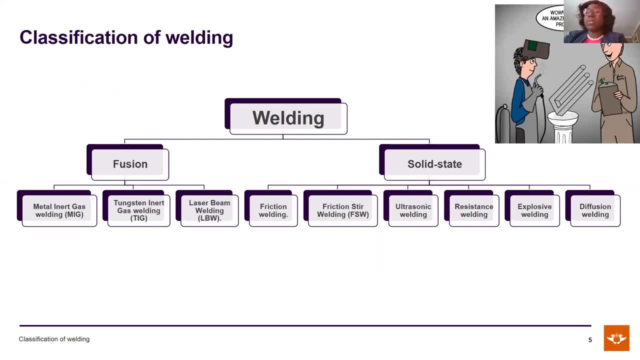 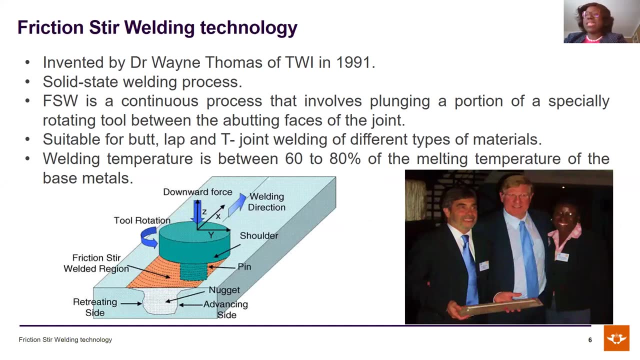 and under the solid-state welding, where we have the friction-steer welding, we also have other welding technologies like the friction welding, the ultrasonic welding, resistance welding and so on and so forth. Now, narrowing down to the friction-steer welding technology that I have been able to, 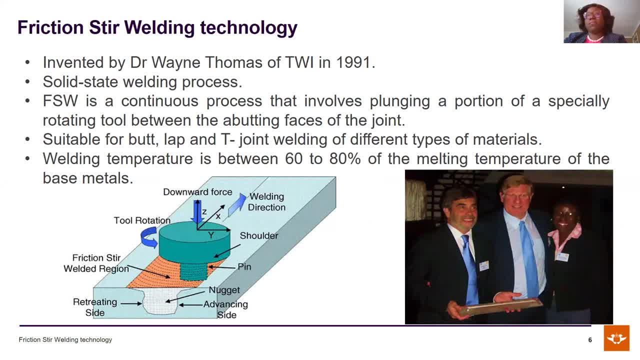 work on and contributed in the last say. I've been working on the field of friction-steer welding since 2008,, where it lasted 12, 13 years. This technology was invented by Dr Wayne Thomas of the Welding Institute in the UK in 1991.. It is a solid-state welding technology. 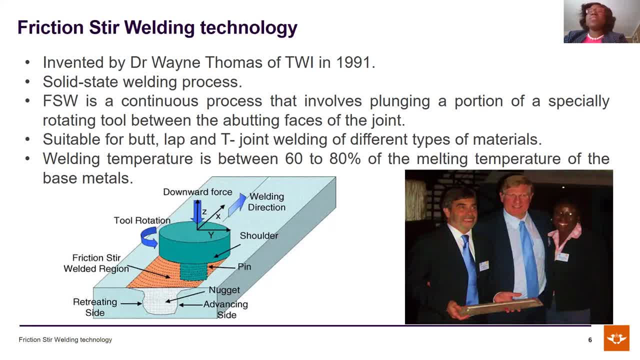 and it has been used in the welding process. as I mentioned earlier on, It's a process wherein we plunge a tool into two abutting faces of two materials to be joined. The materials could be similar and they could be dissimilar. This technology has been used to join metals. 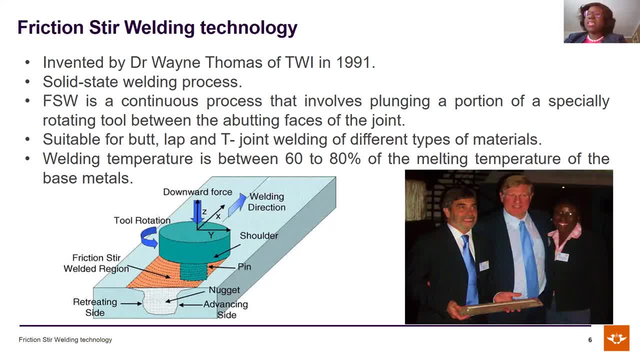 plastics and composites as well. Over the years the technology has had a lot of improvement. It is suitable for BAT, LAB, T-joint and so many other joint configurations. The welding temperature is usually between 60 to 80 percent of the melting temperature of the base materials. 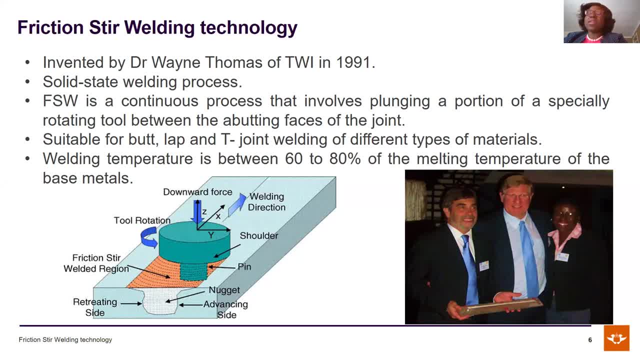 I recall when I have performed welds using the friction-steer welding technologies, I've had the opportunity of wearing a T-joint. I've been able to do that for a long time. I've been able to do that for a long time. I've been able to do that for a long time. 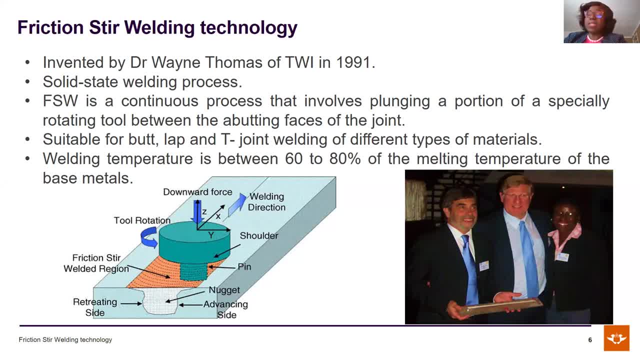 What are the interplay between его saline sun-combination technologies using your own materials? Well, I think that's interesting. I am very familiar with the biochemicals of people In need of biochemical saline, biochemical materials. I have exploring some reservoirs around the globe, including from so many different countries. Why do you think? 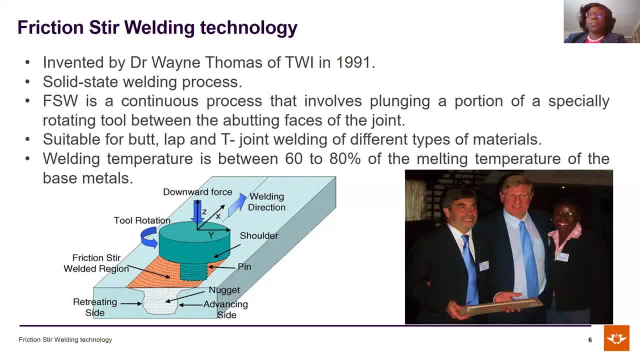 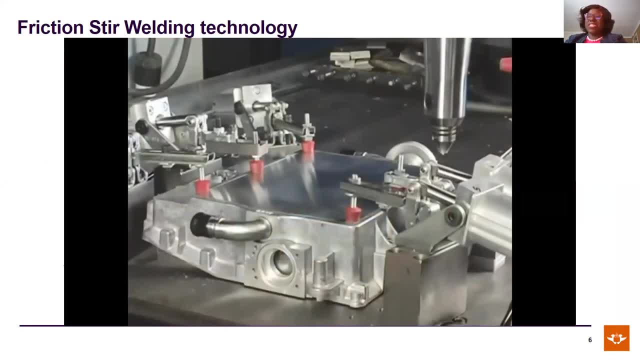 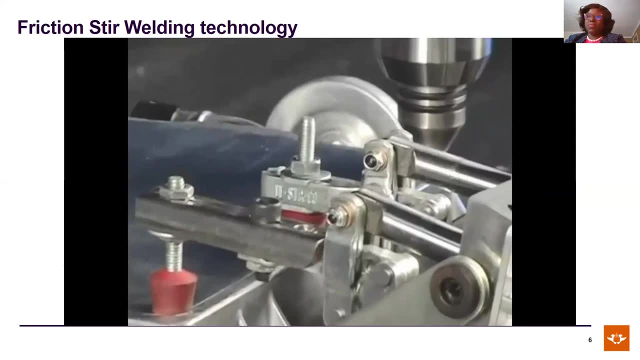 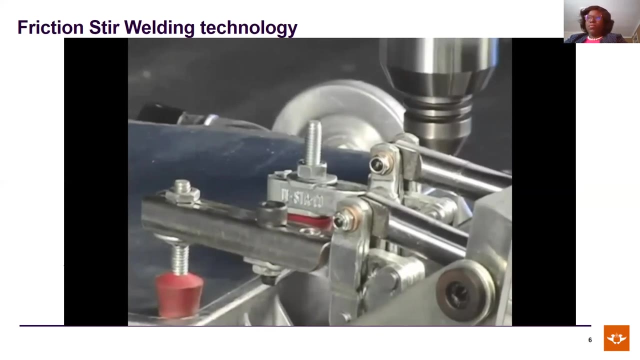 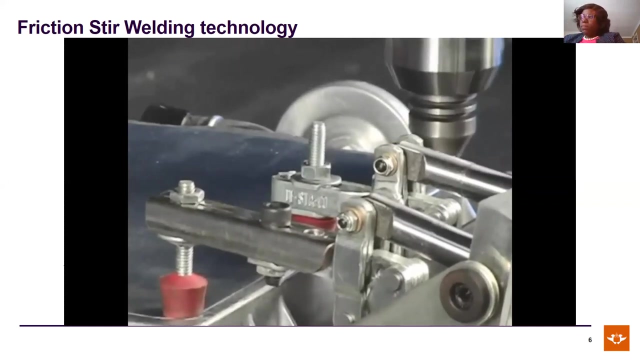 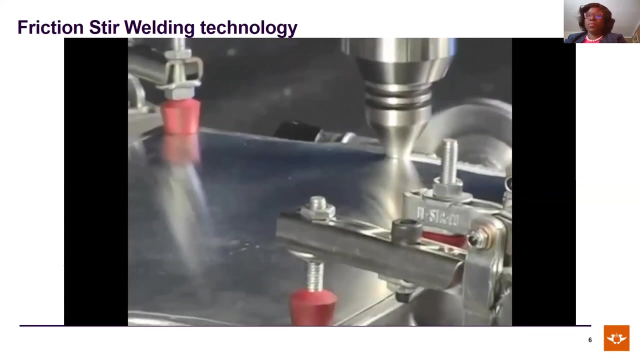 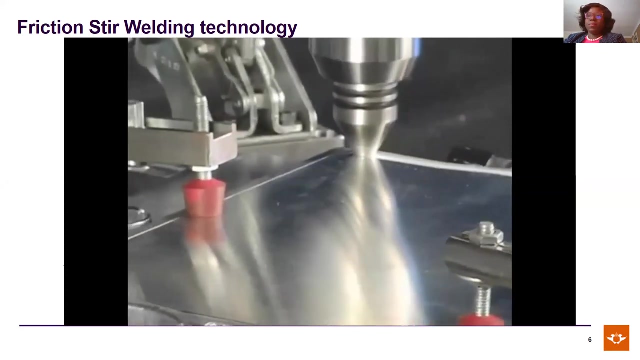 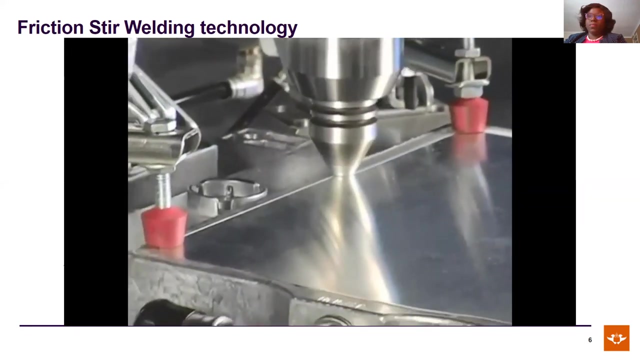 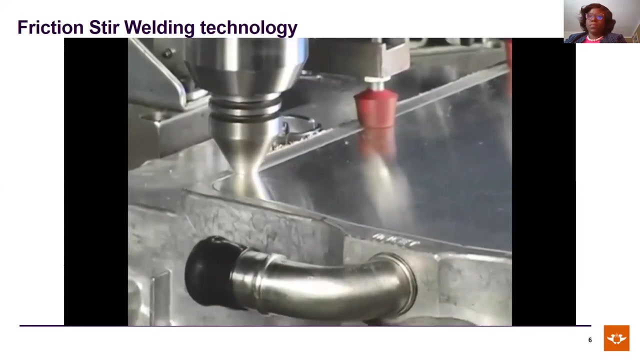 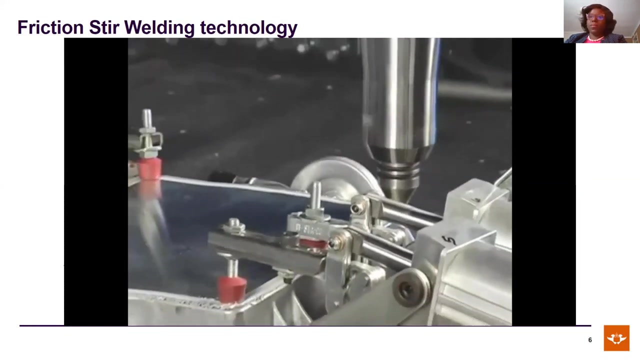 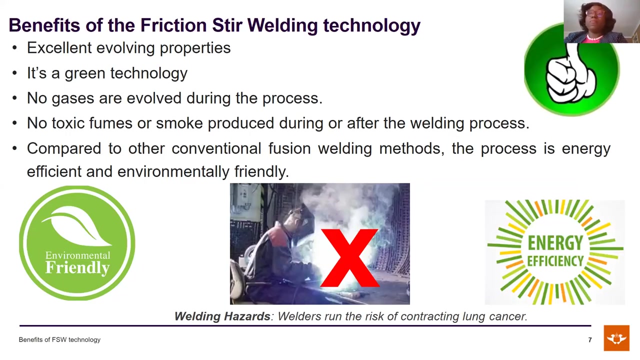 we should find ways to find them, Because nowadays pieces ARMED being joined. Thank you, That was a video showing, just for people to understand better, the efficient cell welding technology. It's been used in selling of engine blocks, So, furthermore, the technology has proven to be highly beneficial. 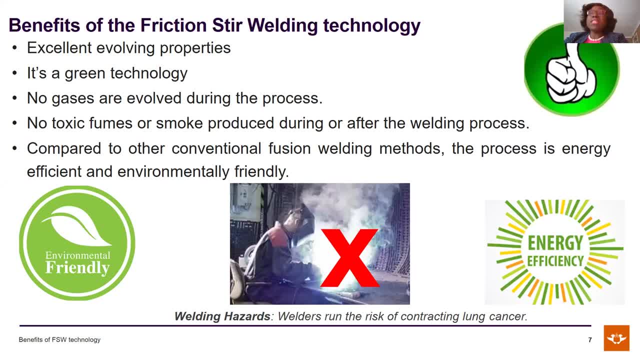 for the people who are using it. To the industry, in the sense that it enhances the evolving properties of the welds, are far better when compared to the conventional welding technologies. It can be referred to as a green technology In the sense that during the welding process, 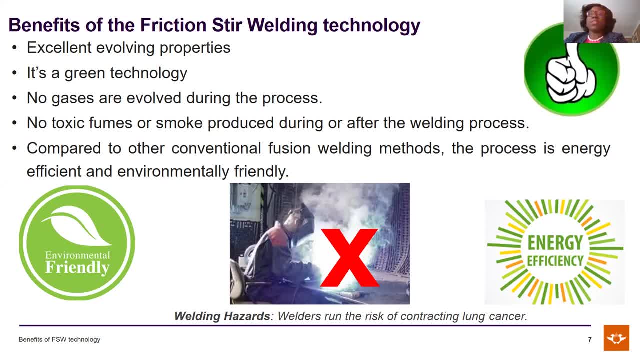 there's no film that is given off during the process, No gases are evolved during the process And you Do not even need a nose mask. I can tell you that, Yeah Well, all the For all welds I've had to pay for on efficient steel welding machine. 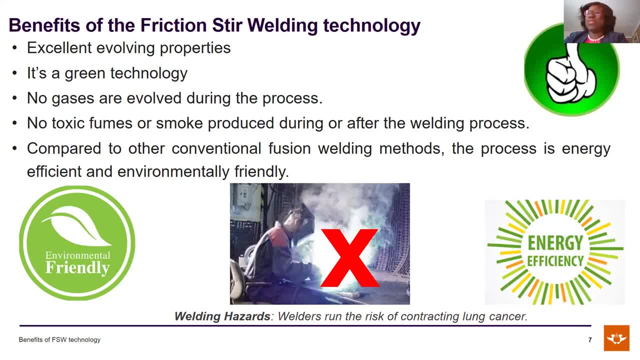 I do not have to use a nose mask, as it is today with COVID-19.. But we use eye goggles in case of debris that could fly off during the welding technology. So no toxic films or smoke is produced during the welding process And hence, when compared to other conventional 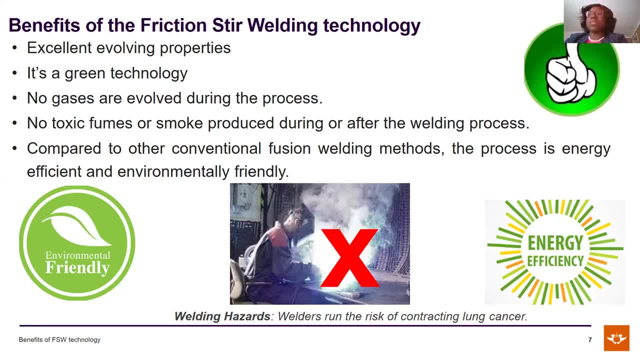 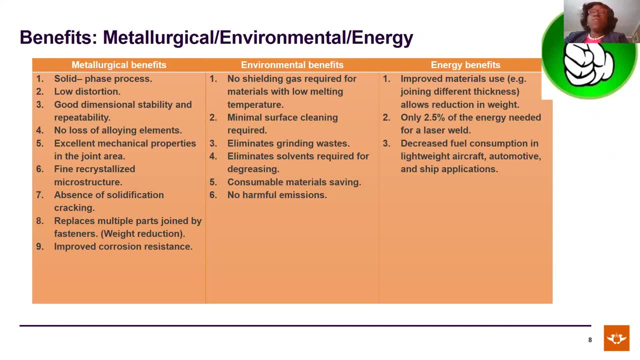 fusion welding technologies. it can be said that the fusion steel welding process is highly efficient and environmentally friendly as well. Furthermore, to still benefit, furthermore there are from the literature and also from what I have experienced in working with this particular technology. the technology comes with enormous benefits. 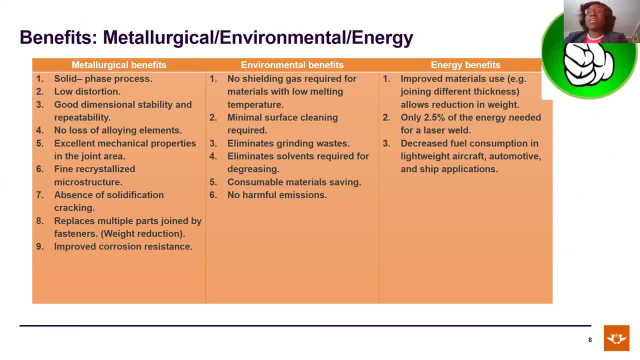 Regarding metallurgical benefits, environmental benefits and energy benefits as well. So it has low distortion, good dimensional stability, absence of solidification and cracking, as very common with the conventional welding technologies, And for environmental benefit as well- huge as well. No, there's no need for shielding gas. no smoke eliminates grinding waste and all of that. 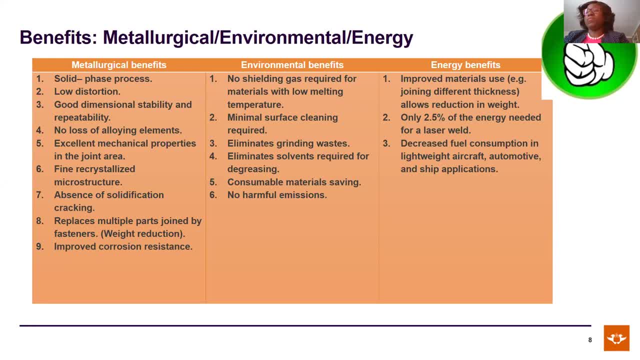 And it's also beneficial. It has energy benefits. Yeah, There are also a lot of benefits as well, In that it has The materials can be used, can be Can have a Can have improved material use And it has been proven in the aerospace industry that this technology has led to decrease the fuel. 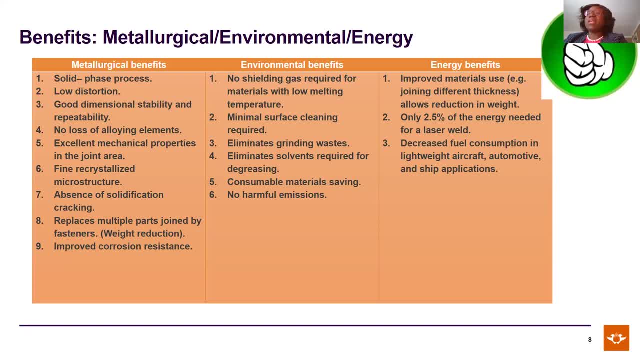 consumption. in lightweight aircraft, Wearing rivets have been replaced with fusion steel welding And that led to To reduce the fuel consumption. To reduce the fuel consumption, to reducing the weight of the aircraft And, with the reduction in the weight of the aircraft, 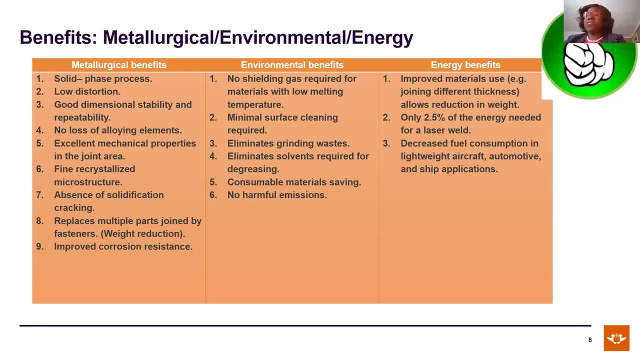 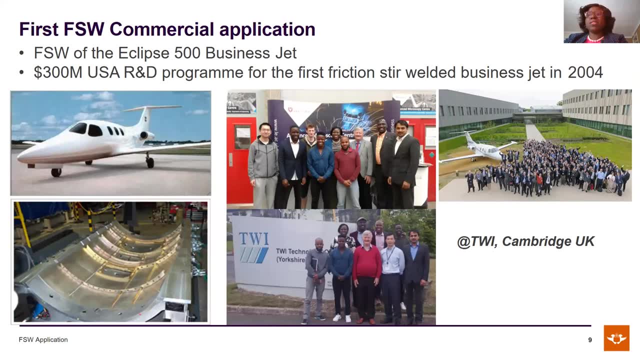 that led to a decrease in the fuel consumption. The first Russian steel welding commercial application was conducted in the year 2004.. And this was tagged as Eclipse 500 business jet, as seen at the left hand corner of my slide. This was a USA research and development program. 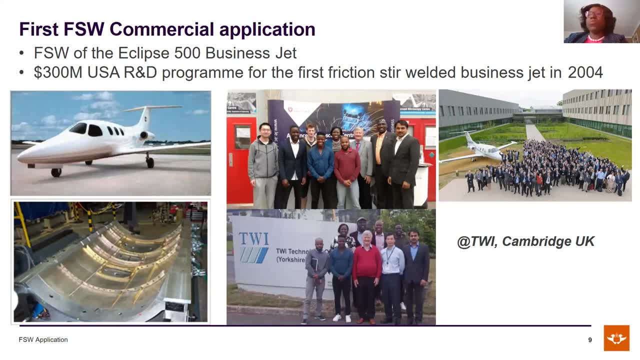 for the first Russian steel welding commercial application, which cost the US government $300 million, And this was done in collaboration with the Welding Institute in the UK. I have been privileged to work on collaborative projects with the Welding Institute in Cambridge. The pictures you have there. 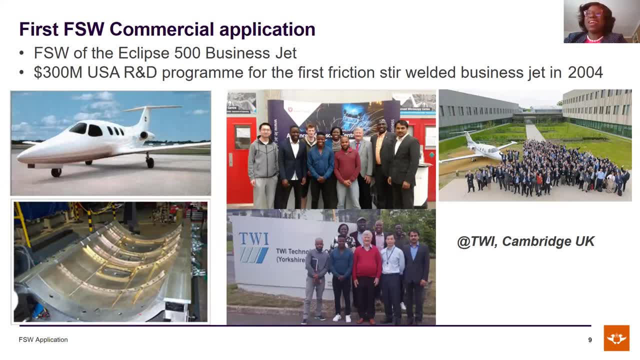 you should look very well, very closely. You will see me there somewhere in the pictures. These are some of the meetings, workshops, trainings that I have been opportune to do at the Welding Institute, And this particular project was in collaboration. 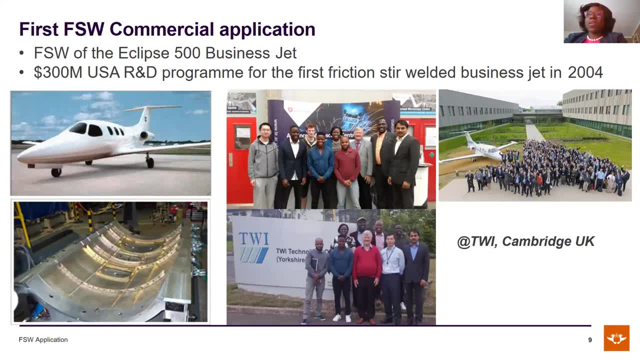 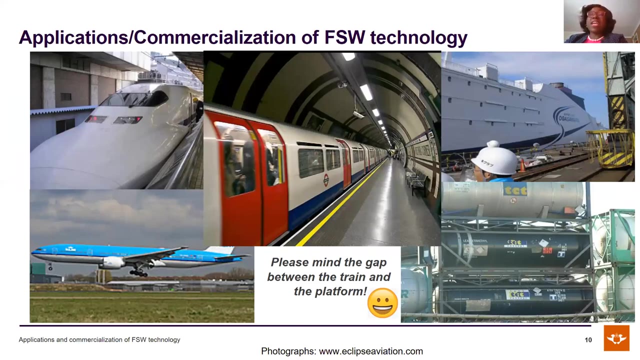 with the University of Leicester, which rounded up March 31st 2020.. I will conclude that the project working, It's industry, academics, industry and a higher educational institution. Further commercialization of the technology today In Shikenshin trains in Japan. 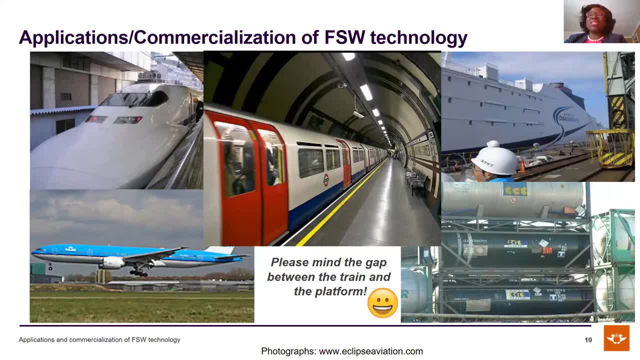 I was opportune to be on the Shikenshin train- That was in 2019,, I recall- And I was looking out for the typical application of the Frictional Steel Welding Technology And my understanding is that the Frictional Steel Welding Technology 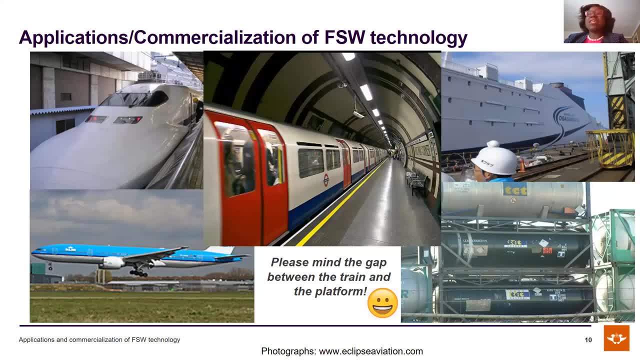 and my understanding is that the Frictional Steel Welding Technology and my understanding is that the Frictional Steel Welding Technology has been used over many years in Japan to weld the floor panels of the Shikenshin Train. This is high speed train that goes. 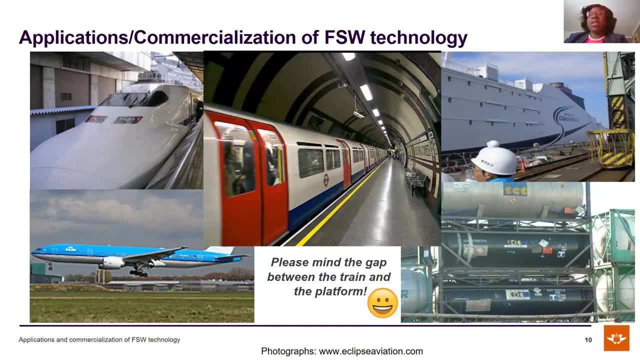 at about 320 kilometers per hour And this technology has been deployed and used because of its and advantages- Stable, low distortion, and all of that. It's been used in the aerospace industry, Like I mentioned earlier, on so many aeros, many of the cruise. 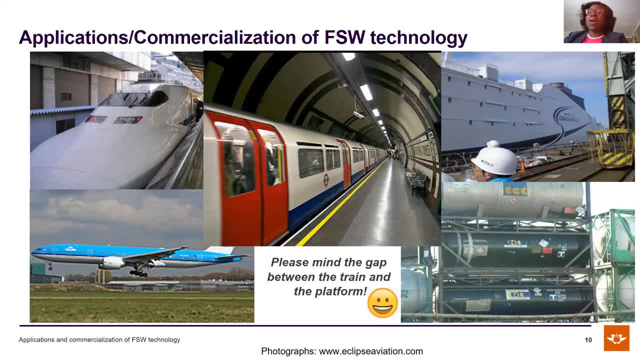 of the aerospace parts. the wings wearing their rivets have been replaced with friction steel welding technology with friction steel welds. Also, some parts on the seats, the aircraft seat brackets, have also been friction steel welding technology has also been employed. 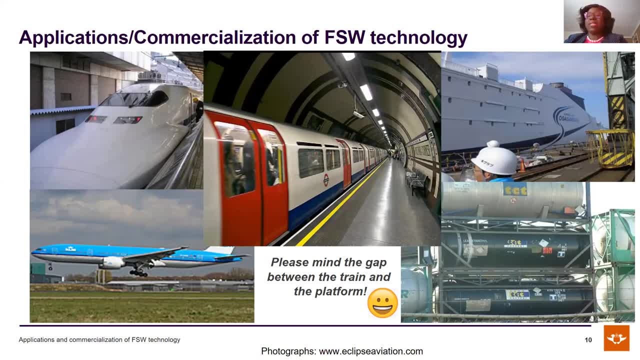 by Boeing to weld seat brackets on planes, And there are some other typical components as well that are patented. where friction steel welding technology has been used on the aircraft, That's also been used on the floor panels of the underground tubes in London. So like I was making a joke that when, as an engineer, 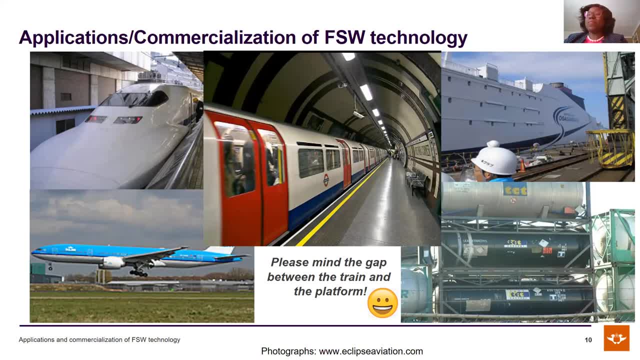 and with the knowledge of friction steel welding technology when I got to know that all the floor panels of the underground tubes in London were produced using friction steel welding technology. So when I go- the last time I was in London and I was going on the train- 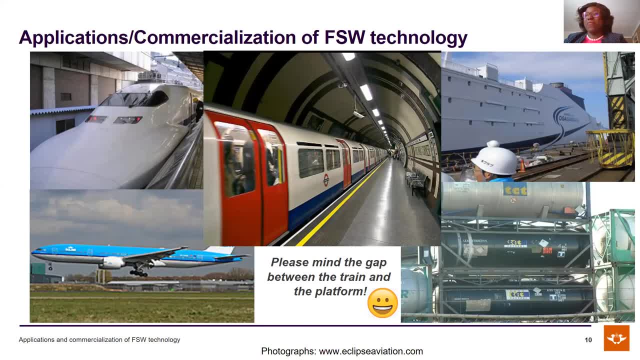 and I was hearing: please mind the gap between the train and the platform. In my mind, I was telling myself that the floor of what I'm getting onto now got friction steel welding welding over there. So other applications include, for example, 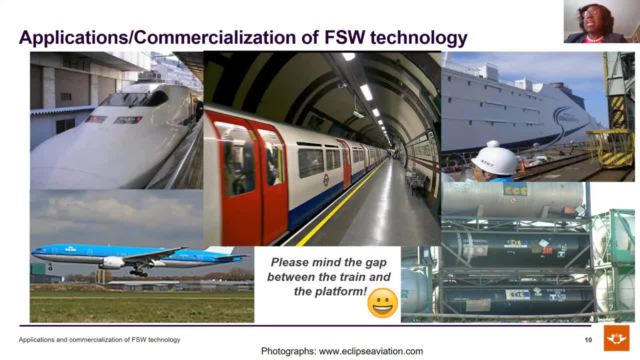 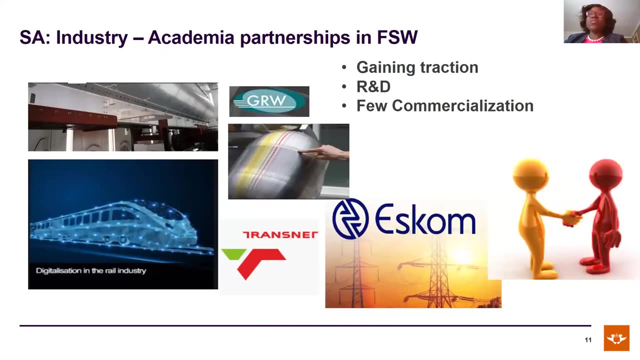 even when we think about, for example, for competition, include shipbuilding in Japan and also in China, We've used official cell welding technology widely on shipbuilding and also in the tank container industries as well. I just want to share a little glimpse. 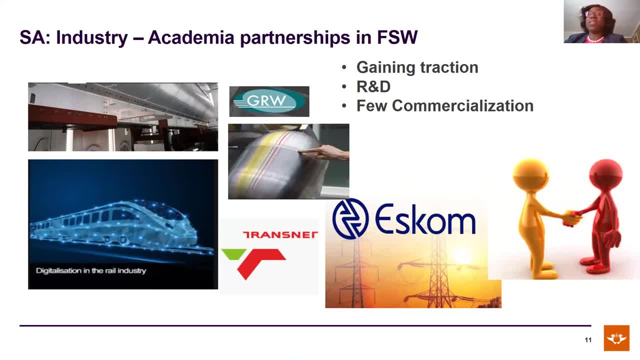 into how far we are in South Africa and on the African continent. Without doubt, South Africa is in the forefront of championing official technology on the African continent And I think most of the platforms at the moment are still only in South Africa. I am aware of some other countries. 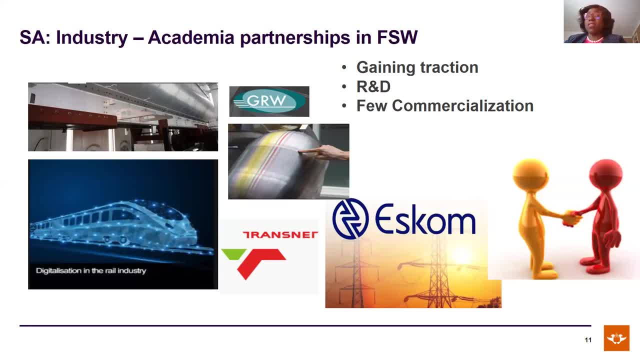 trying to also have interest in the technology, And in South Africa we have some industries are beginning to have interest in the use of official steel welding technology And one of them is ESCOM. that has also sponsored a project that I've worked on. 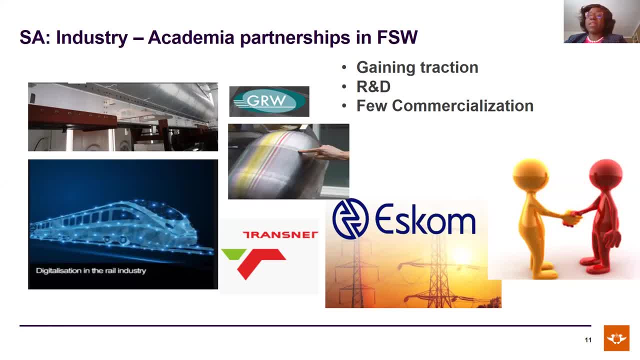 We have Transnet. I've also worked with Transnet as well in the rail industry. ESCOM is the power producing company of South Africa. There's also a tank container industry in Cape Town called GRW. They have been using official steel welding technology. 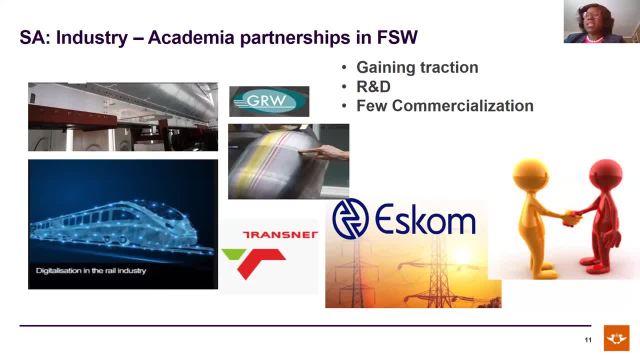 as well over many years. So it's detailed, It's technology, Even though well advanced in Europe. I know that India is also in the forefront of championing so many applications in the field of official steel welding For us in Africa. we are getting there. 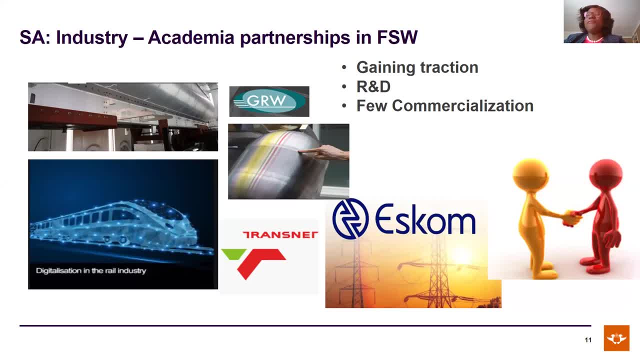 It's getting traction: a lot of research and development projects and very few commercializations of the technology that has taken place on the African continent. I have so many collaborators in the field of official steel welding in India, Like IISC Bank, IISC Bangalore with Prof Satish. 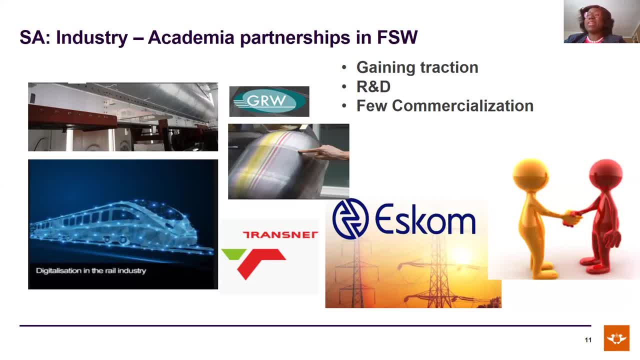 I also have Professor Pal and Prof Majumda in IIT Kharagpur. I've been to these places in India and I have collaborated widely with these two distinguished professors in the field of official steel welding And I'm also very happy with the way the official steel welding 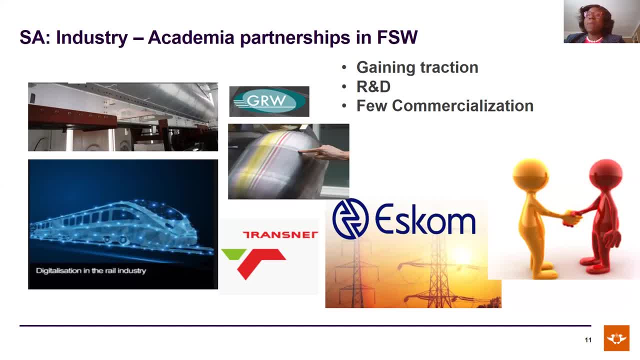 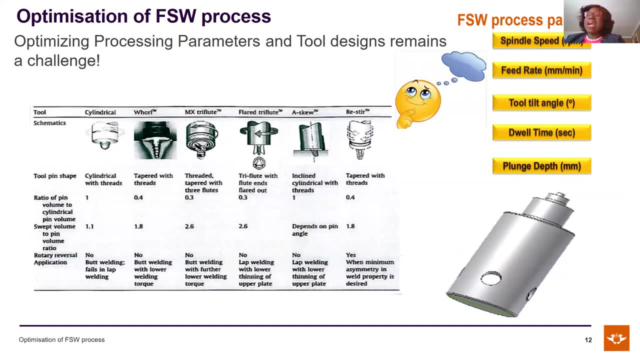 platforms because of the huge cost. I'm happy. I'm happy with so many platforms in India that have been reconfigured from milling machines and they are doing very, very, very well. So I will now move on now to ascertain joint integrities. 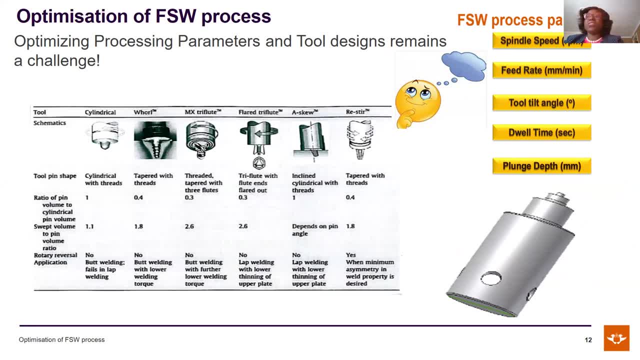 There is a need to optimize the official steel welding process, And this could be quite complex in the sense that there are so many parameters. I'm happy with so many platforms in India, So I will now move on now to ascertain joint integrities. There is a need to optimize the official steel welding process, And this could be quite complex in the sense that there are so many parameters. I'm happy with so many platforms in India, and I'm also very happy with so many platforms in India. 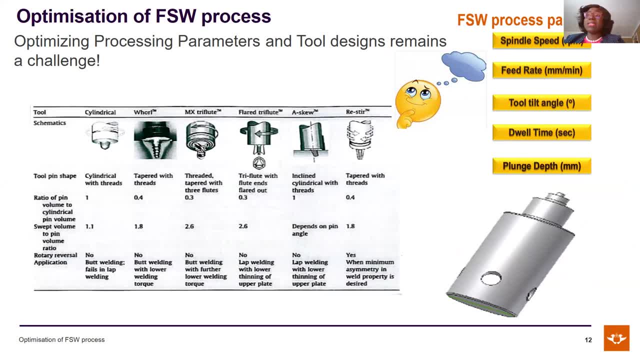 and I'm also very happy with so many platforms in India that need to come to play, considering the official steel welding processing parameters- the spindle speed, the feed rate, the plunge depth, dwell time, the tool rotational speed- and all of that needs to be optimized. 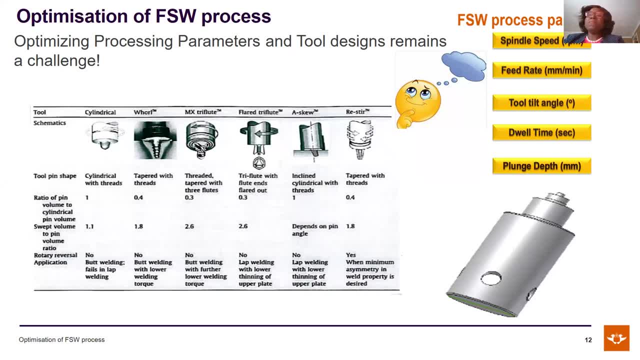 So also the tool designs. There have been so many types of tool designs. The common ones are what I have here, the cylindrical tool with threads, the one- also without trade you want to, the tri-float, the flat tri-float, tri-float, the. 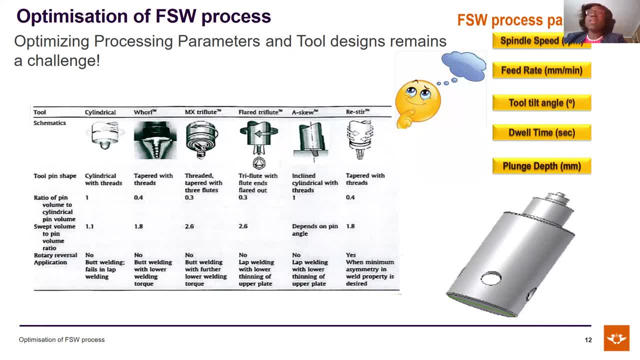 skew and then the wrist. here i recall that one of my students some years ago also designed a tool which we're actually trying to patent at that particular point in time, i recall, which we also use to produce some, some wealth, and it actually gave very good uh flow of the. 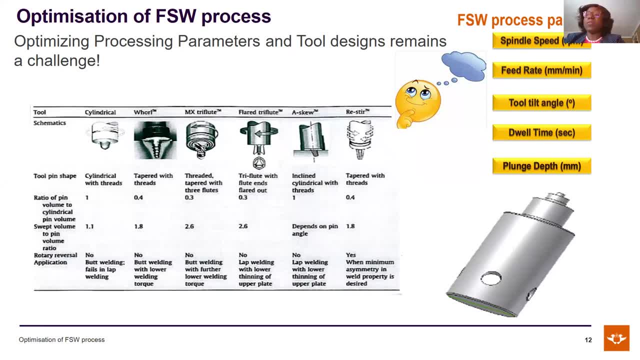 of the materials being joined performed really well. so there are still a lot of research being conducted in trying to optimize the process, and this- the optimization of the process parameters and the tool design- still remains a challenge in fusion steel welding. but then we are getting getting there, and this aspect as well speaks directly to the joint integrity. the point is that 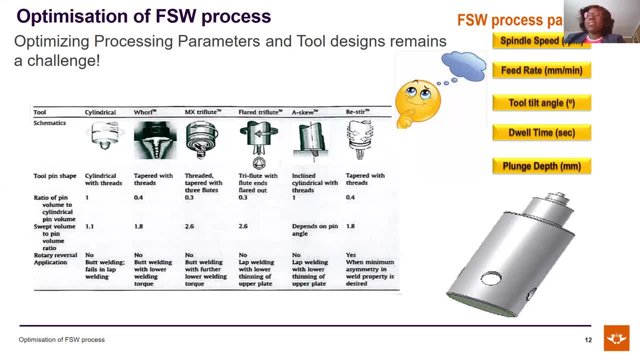 we cannot be talking about characterizing, having a good world materials characterization- without, first of all, understanding the basic rudiments that needs to be put into place, and then we have to understand the basic rudiments that needs to be put into place, and then we have to understand the basic rudiments that needs to be put into place. 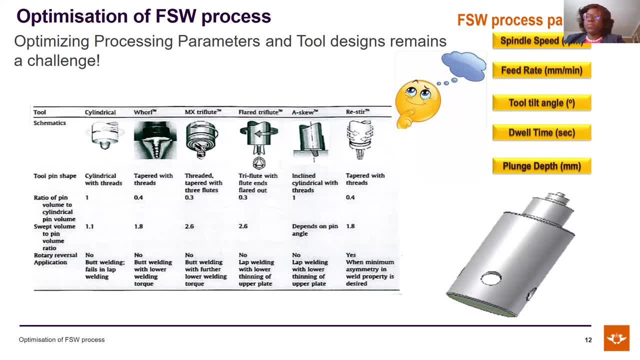 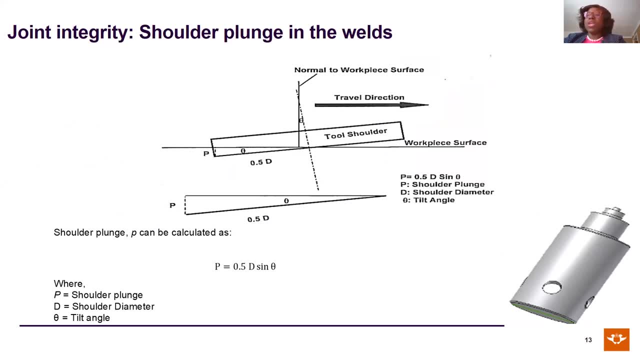 in optimizing the future steel welding process first. other aspect that needs uh to to be done to improve the joint integrity of of friction stairwells is optimizing the shoulder plunge in the in the well during the welding process, and this is uh can be explained through the calculation that i've 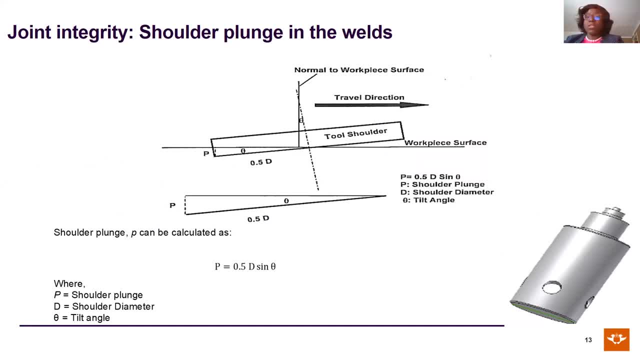 i have on the screen now, wherein we calculate the shoulder plunge, which is a 0.5 of d sine theta, where d is the shoulder diameter that is being used, the shoulder diameter of the tool pin that is being used to produce the world, and then theta, that is the two, the two tilt angle that is being 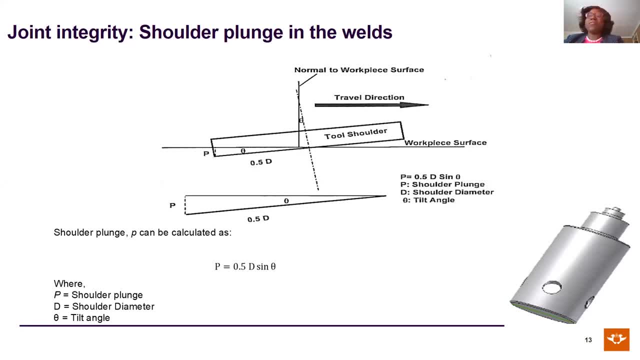 used to produce the world. this is to give a rough idea, an estimate of how much we should plunge our tool into the world during the welding, because these tools shoulder helps with the consolidation of the of the of the worlds. it helps with enhancing the materials flow, the material flow. 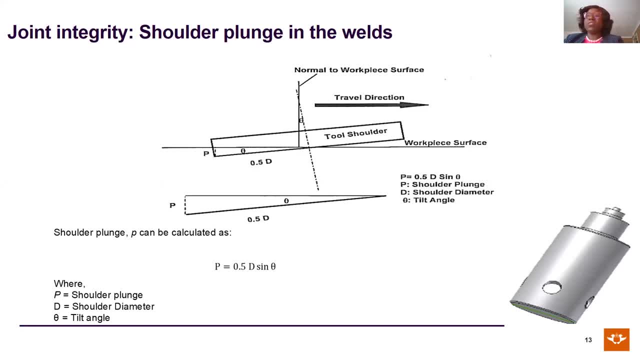 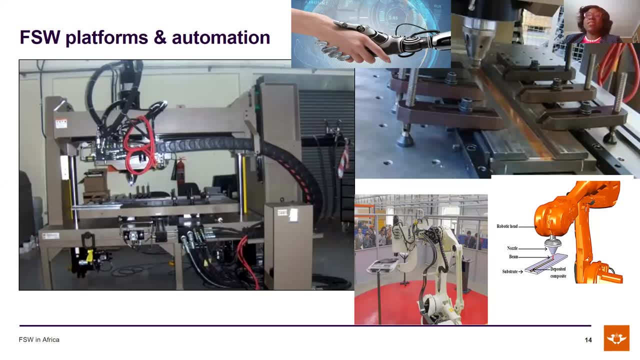 during the welding process. hence this also has to be optimized. on this particular slide i've shown uh future set where the platforms and automation the process has been fully automated. today there are so many uh robotic facilitated welding technology. they've been put out of the work a lot. i've also shown here that residual Algunca Ale Nalade dep�도 aим. 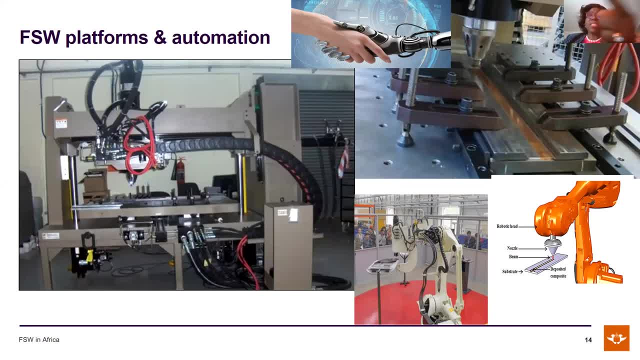 making platforms across the globe, and the one on the left hand side here, uh, that is the official, still welding platform. that, uh, that's we have always used, which is at the nancy mandela university at port elizabeth, where i did my doctorate here in south africa, and the other 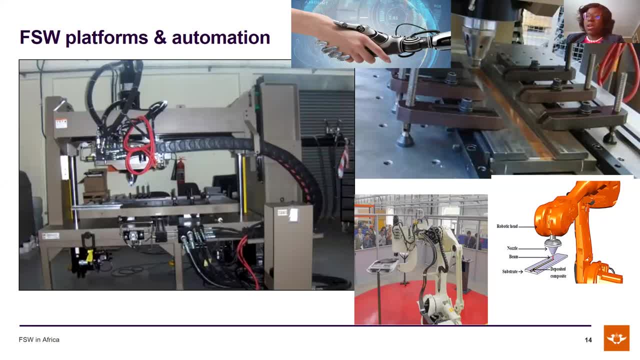 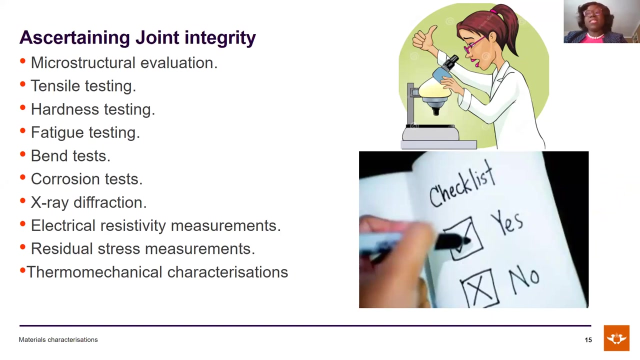 uh, robotic. uh, the robotic efficiency welding platform you have down at the at the bottom right hand corner of my slide. this picture was taken at the twi in the uk, so the process is fully automated and it's? uh has been used in various applications today, so a certain joint integrity. 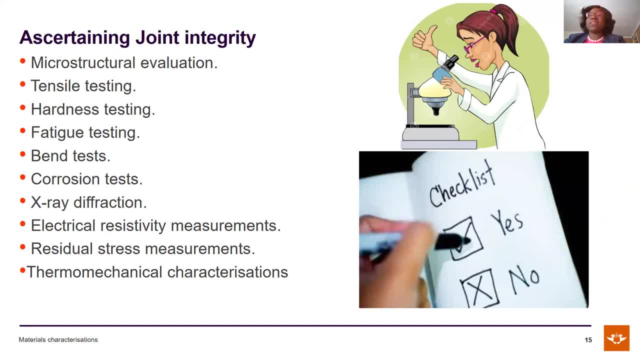 i've listed here a couple of uh materials characterizations that uh that can be conducted. this list is inexhaustive. i say inexhaustive is exhaustive because the wells that we are, we we producing, has typical application. so the materials characterizations that a researcher wants to do. 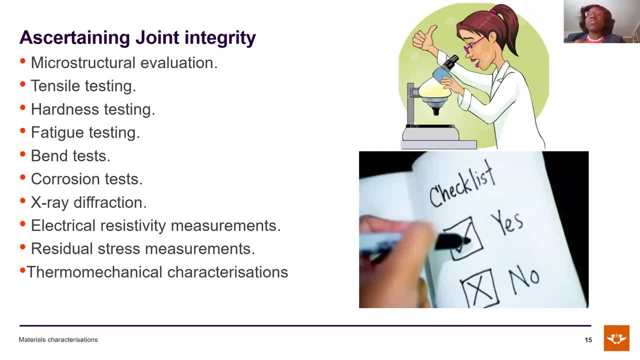 at any point in time will always speak to the typical application of that particular well. but then there are general guide, rule guidelines, general general, and i will slash with basic materials. characterizations that should be conducted when we are, when we are producing wealth like the first three are very, very basic. 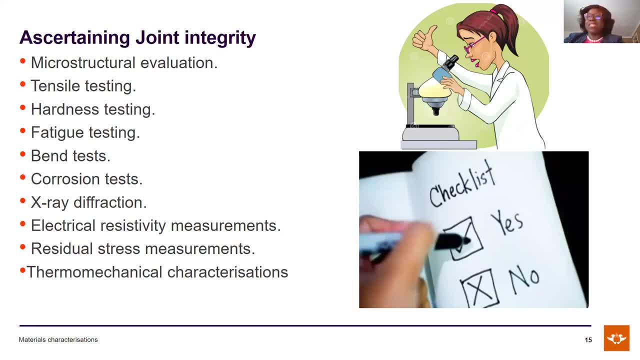 the microstructural evaluation, tensor testing and hardness testing. these three are very basic and they are our first points of call that we always need to to to consider when we produce our wells, to be able to see or know what is happening in the world in order to ascertain the joint. 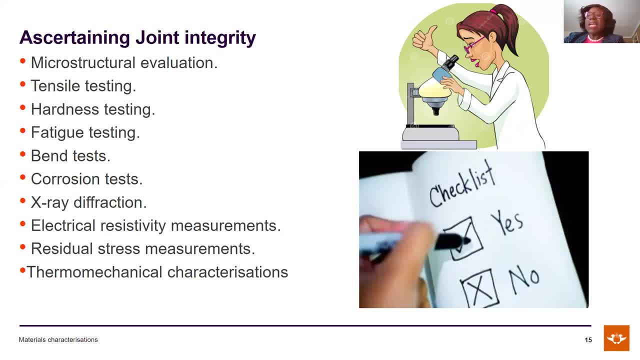 integrity. And then the checklist. a checklist needs to be built by the researcher. If a particular world will be used in applications wherein fatigue will come to bear, fatigue testing needs to be conducted. Then the researcher also needs to determine when burn tests are. 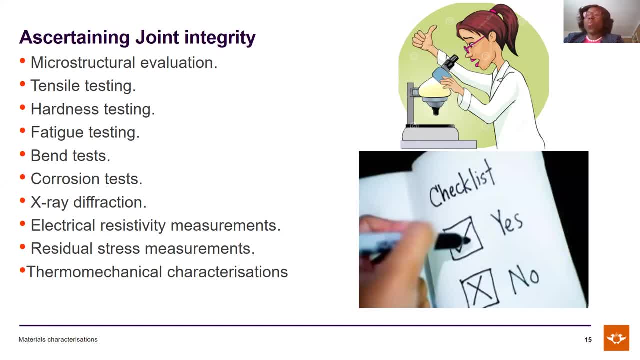 required when corrosion tests are required with respect to wells that will be exposed to various atmospheric temperature, some environmental conditions and all of that. The S-ray diffraction can be considered electrical resistivity measurement when it has electrical applications, residual stress measurement, thermo-mechanical characterization- This list is inexhaustible. 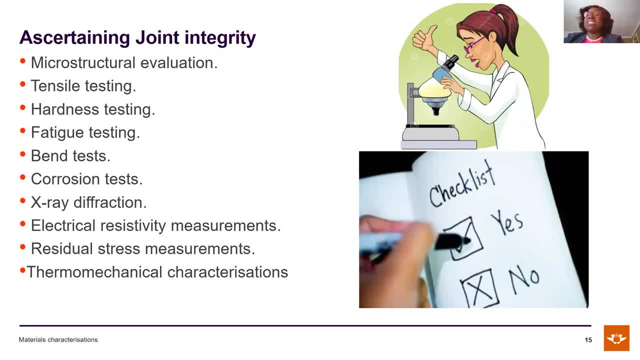 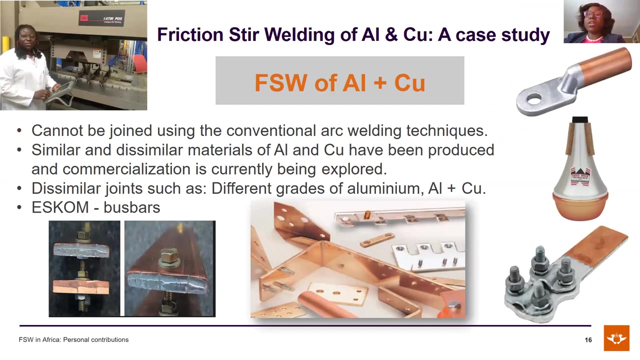 There are so many other materials, characterization techniques, There are so many other materials that have been developed today that are applicable to wells. All we are trying to do is to ascertain the joint integrity of the wells that have been produced. So I will now go ahead to shed a few lights on a case study of fusion cell welding, of 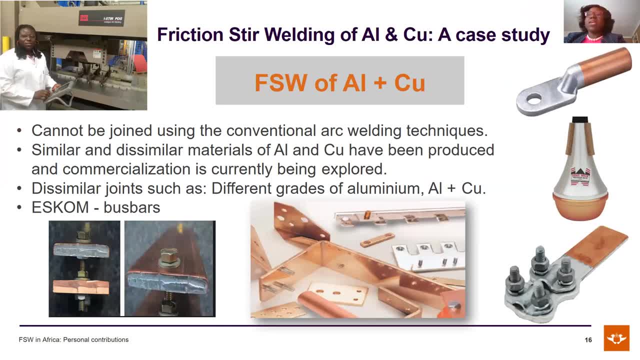 aluminum and copper that I have been involved in. Aluminum and copper finds application in balls bars in the electrical system. Okay, So this is a case study of fusion cell welding of aluminum and copper, and this project was sponsored over many years by ESCOMP, which is a power generating company in South Africa. 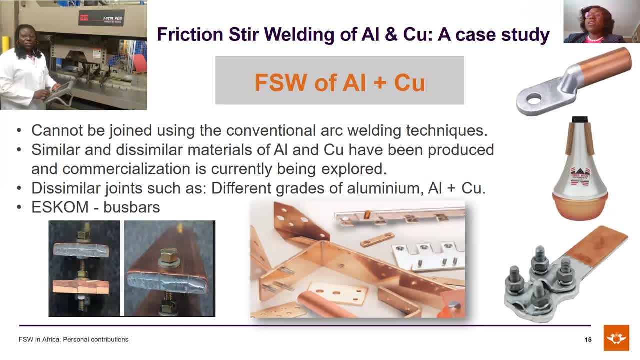 The fact still remains that, up to today, these two materials, even though they come with huge benefit, they cannot be joined with conventional arc welding techniques. Hence the application of solid-state welding technology, like fusion cell welding that has been considered to. 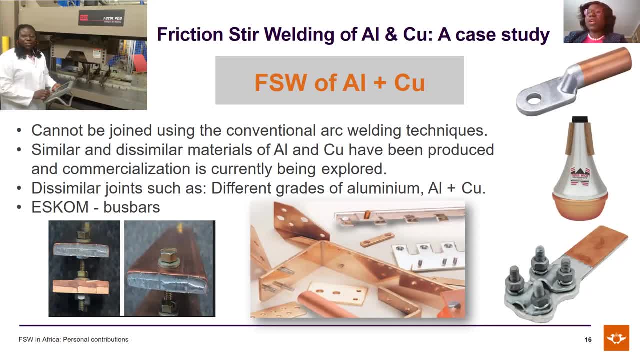 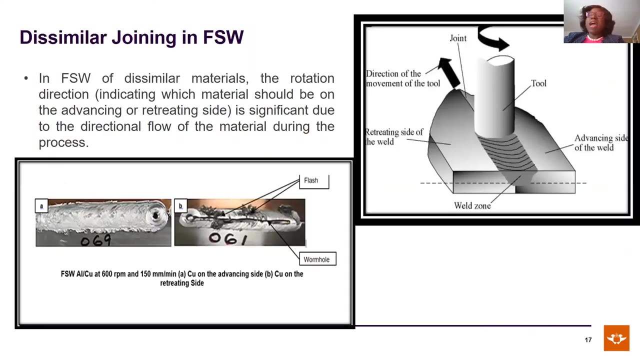 join the two materials either in aluminum or copper. So in this particular field a lot of research has been conducted, from myself and some of my research team members, So I would like to mention some rudiments to joining dissimilar materials using the. 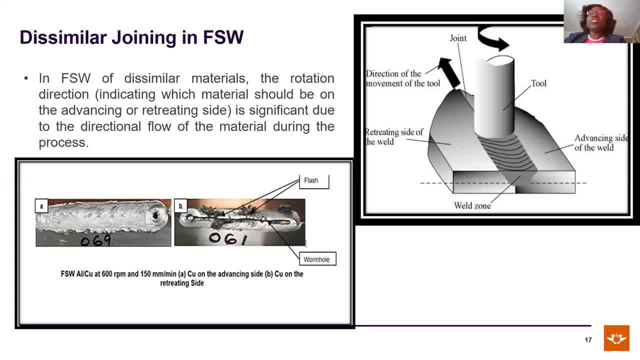 fusion cell welding technology. The position of the tool during the welding process is very, very key and very important. So at the beginning, in dissimilar joining, researchers were not aware of where to actually place the material and also the direction of the tool as well. So I did a fundamental 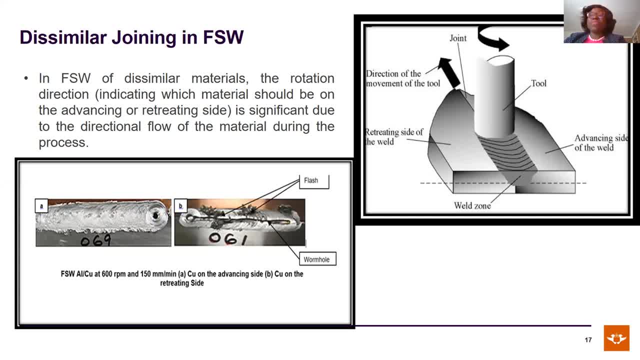 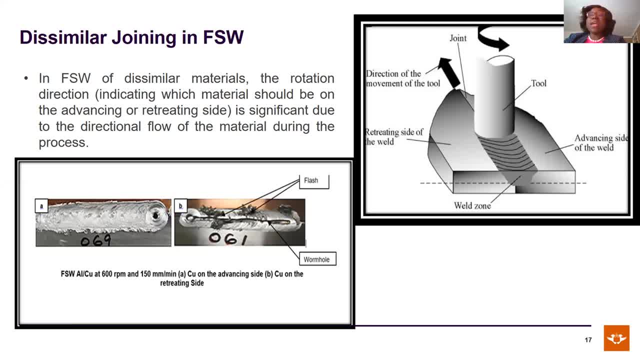 and so there remained no rates, both in general and in foreign market place, went up. That's right, Because we have two dissimilar materials. so in the case of copper we are in another case of BROWN, and in other case of copper we are in another case of puisqu. it started. 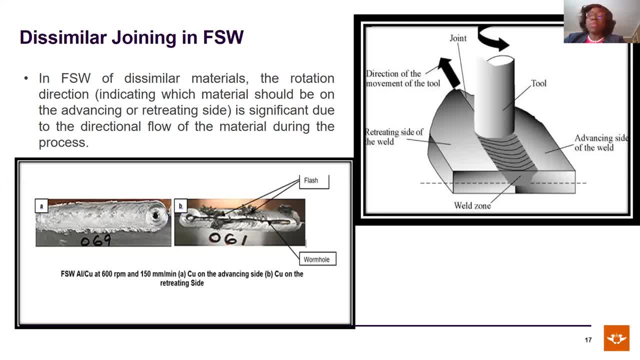 going down in terms of what they were called, And therefore the special material is beХlive hein, the weld that I'm showing here. on the left-hand corner of my slide you will see weld 069, which has copper on the advancing side and then aluminum on the retreating side. That 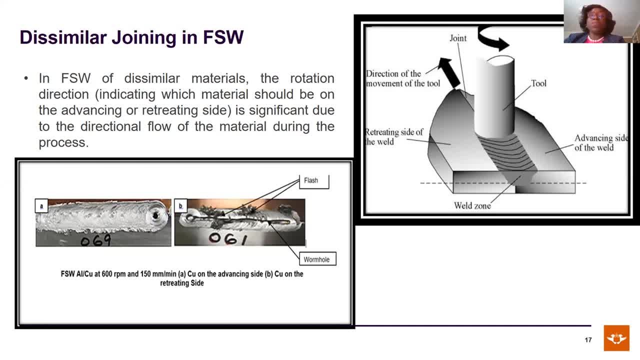 is weld 069.. While on the right-hand side I have placed copper on the retreating side and aluminum on the advancing side. You will visibly see the heavy flash and the wormhole that was produced. Now, this is the basic research in trying to determine where a particular 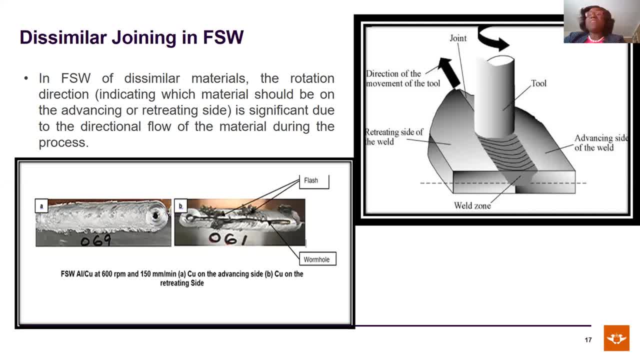 material should be placed. Now from this basic research I did other feather welds as well and then also confirm from other researchers working in the field field of dissimilar crucial steel welding, This particular study has been concluded that when we want to join dissimilar materials, the material with the higher melting point 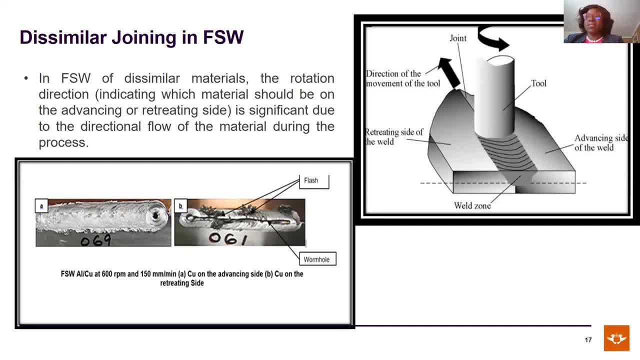 should be placed on the advancing side. The notation of advancing side and retreating side are shown on the schematic diagram that I have on the right-hand side of my slide In dissimilar material joining the rotation direction of the tool and where we place the. 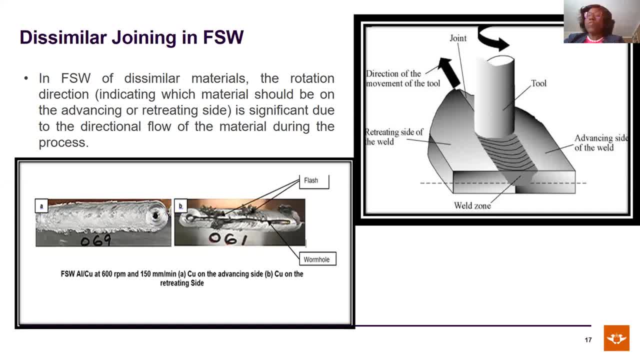 materials is very significant due to the directional flow of the materials being joined during the process. This is a basic, fundamental research which I have published. I've mentioned this in one or two papers. Other researchers have also published this as well. It is expected that other researchers coming along that need to join. 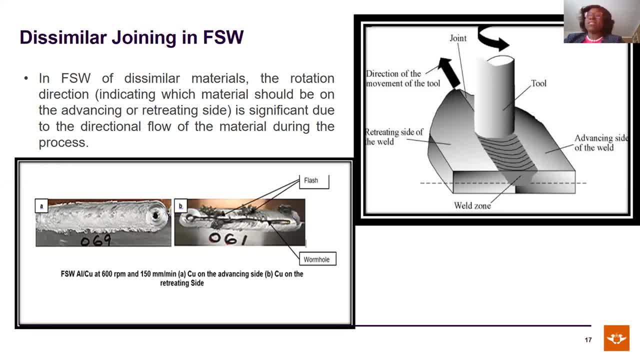 dissimilar materials do not need to go back to the basics of what we have done. This has been a study done and concluded that to enhance joint integrity, to have a good weld, the material with the higher melting point should be placed on the advancing side of the weld. 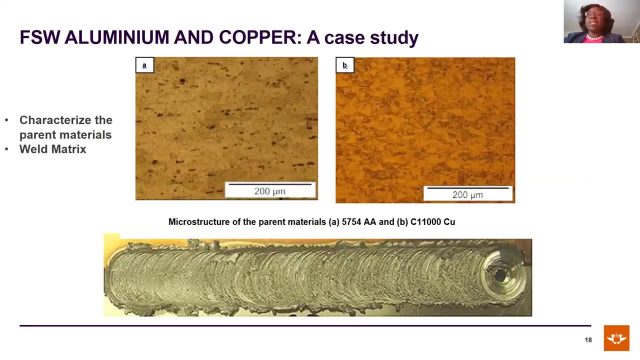 So this is also expected that, for a start, today, in the next, Before it is such that you will go into conducting the welds, it is expected that it is such that you first of all characterize the parent materials, because you need something to benchmark, You need the data on materials as benchmarking for 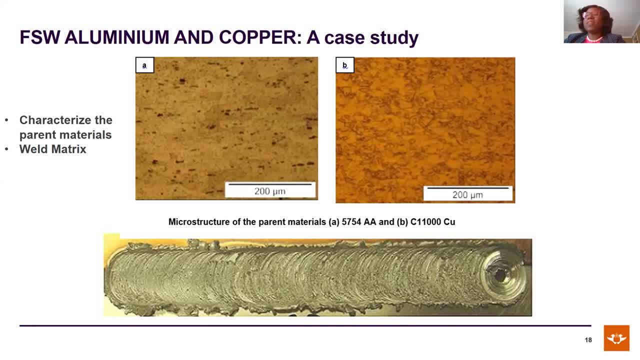 a benchmarking. So when we can Youtube do tourists and your script, You can pull up all of thisул. So when we produce the wells, we then have something to benchmark to the parent materials. So we characterize the parent materials individually. It is also expected that we join first of all. 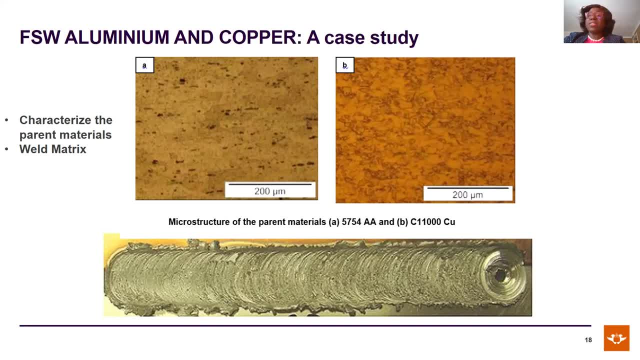 the parent materials as similar materials. For example, when I want to join aluminum to copper, it is the experience of me as a researcher to start by joining aluminum to aluminum of that particular grid that I want to join, to also join copper to copper. 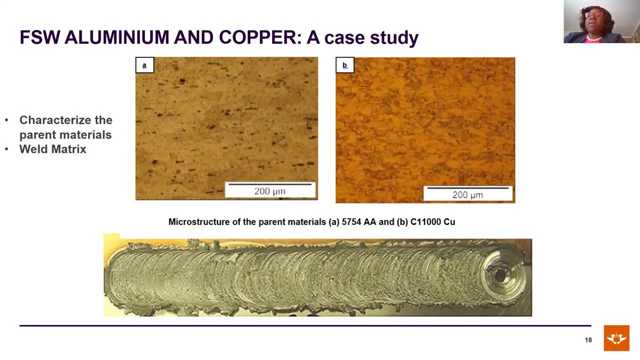 and then, before progressing, to come up with my world metrics. World metrics are usually- it's always- advisable that before we come up with world metrics, that we consult the literature to see what people have done in that particular field of study, And then you can use that as a basic. 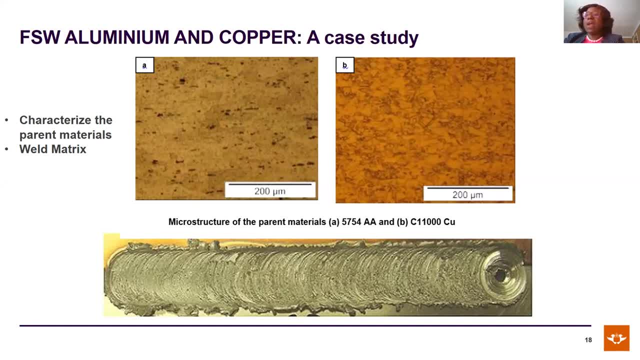 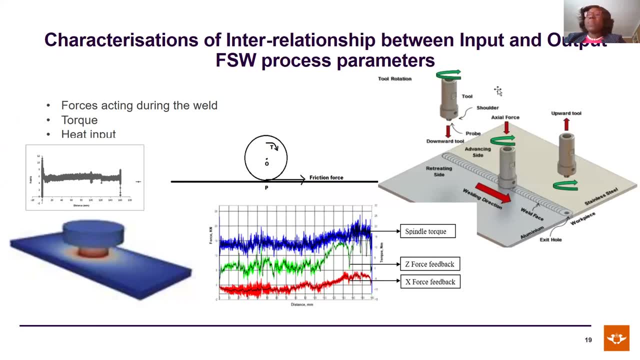 to form your own world metrics to carry on your experiments. It's also important in characterizing wells that we consider the characterizations of the interrelationship between the input and the output. historical writing processing parameters. I mentioned earlier on an earlier slide, the input processing parameters. 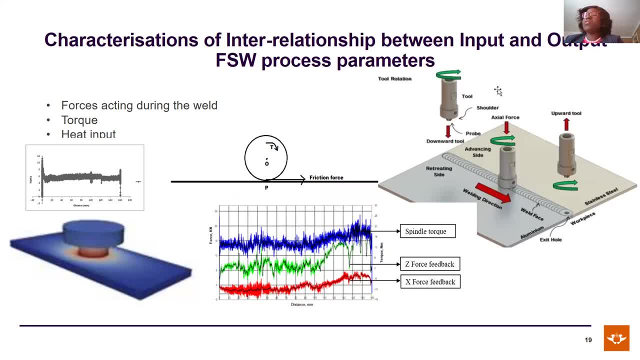 the tool: rotational speed, the feed rate, the net interval parameter, the tool plunge, the tool tilt, angle, the dwell time and a couple of them- I think there are five or six of them- that are basic input processing parameters that we need to enter into the welding computer system. 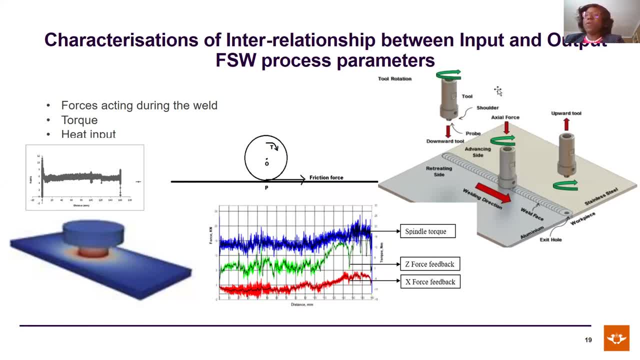 for welds to be performed. After the welds have been performed, a number of friction cell welding machines are able to give some output data. We are able to analyze the forces acting during the weld. We are able to correlate the joint integrity with the forces acting during the weld. 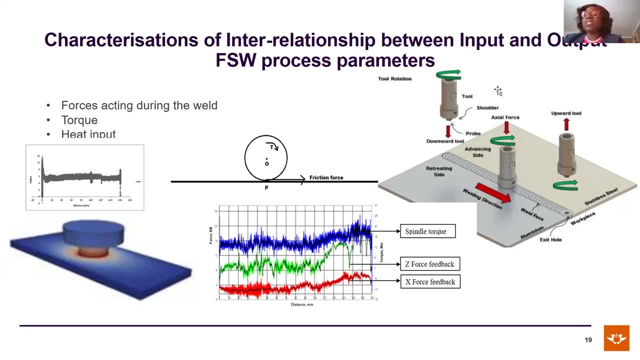 We are also able to have data like torque and then the forces acting for most friction cell welding machines. we have the forces happening in three direction with the X, Y and Z forces. We have the spindle torque data and we are able to analyze the forces acting during the weld. 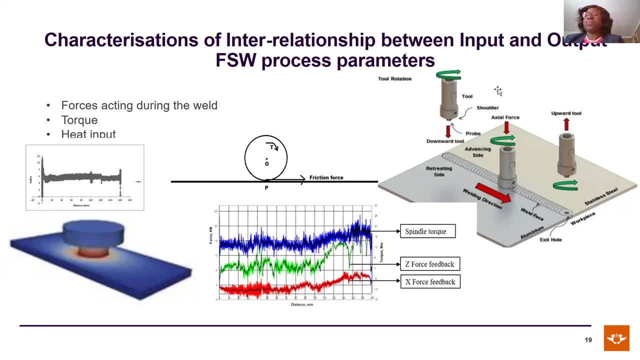 We are also able to calculate the heat input into the weld. The heat input into the weld is a very important parameter as it has been correlated to dictate the quality of the weld. There are formulas that have been used that are available in the literature, to calculate the heat input into the weld. 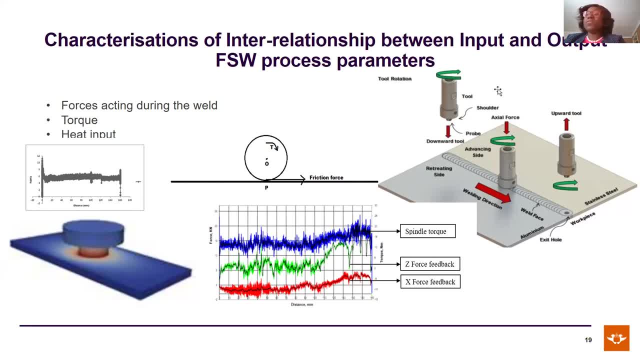 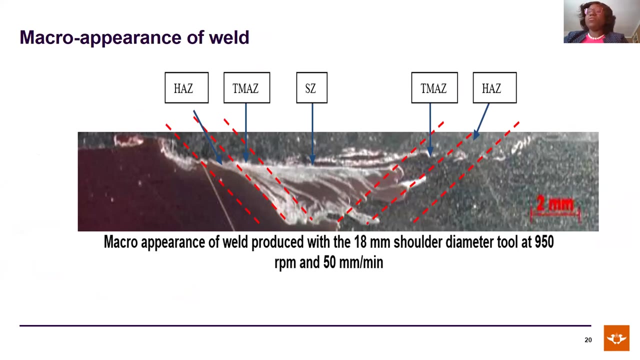 Also, there are so many simulation softwares, mathematical, mathematical relationships and softwares that are available in the literature to calculate heat input, also to be able to estimate the welding temperature during the welds, After having looked at the interrelationship between the input and the output processing parameters. 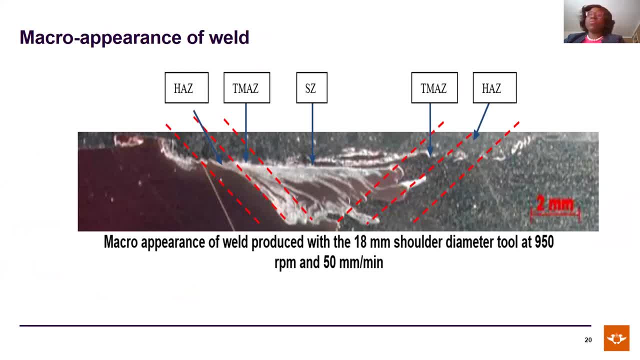 we. it is also expedient to also have the macro application and then the to have the transfer of heat down the weld. Much of the work we have done in the last six years has been focused on the field of low pressure welding, and this has been a very important thing for us to do. 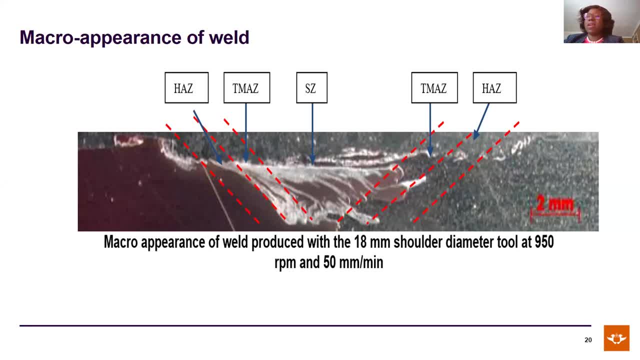 integrity of fission-steer welds as well. I think I recall that one or two papers have been published wherein we highlighted non-destructive techniques, how we have deployed them to ascertain the integrities of fission-steer welds. So we then characterize fission-steer. 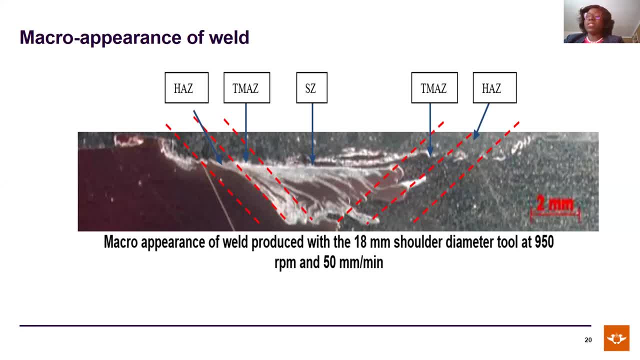 welds into the steer zone, which is the center of the weld where we plunge the tool. That is the point where the tool pin has acted during the weld. Further from the steer zone, we have the thermo-mechanically affected zone and then we have the heat-affected zone. Then, at the extreme, 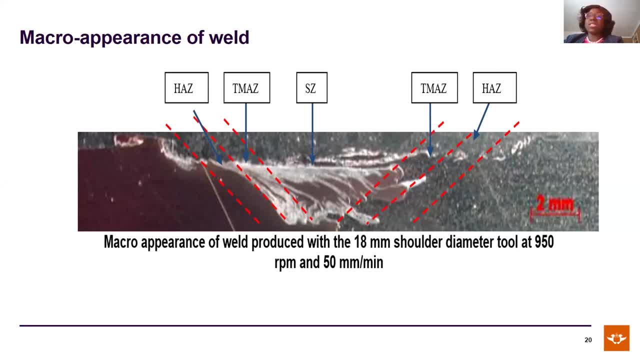 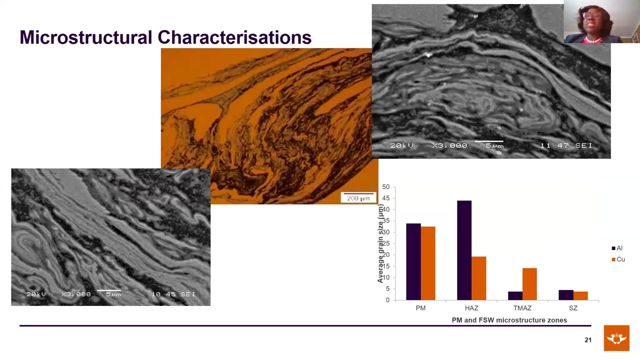 left and right, we have the parent material, as shown in this particular marker. This will enable us to see the flow of the material that has been joined during the process. Further to this, we then consider microstructural characterizations. As you can see, we can start with the use of an optical microscope. 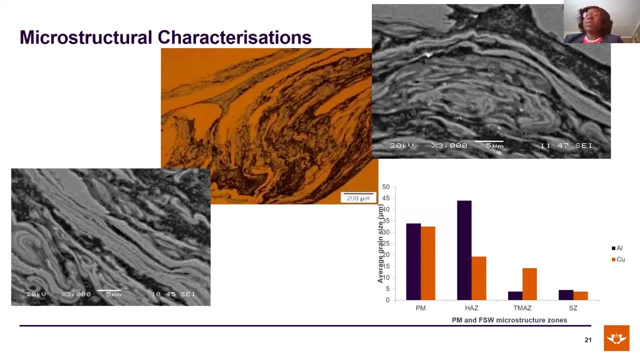 and then progress to the use of SAM. TAM has also been used to characterize microstructural characterizations of fission-steer welds. Under microstructural characterizations we also consider the grain sizes as well. We measure grain sizes because it's expected that the steer zone will always have very refined grain sizes if our processing 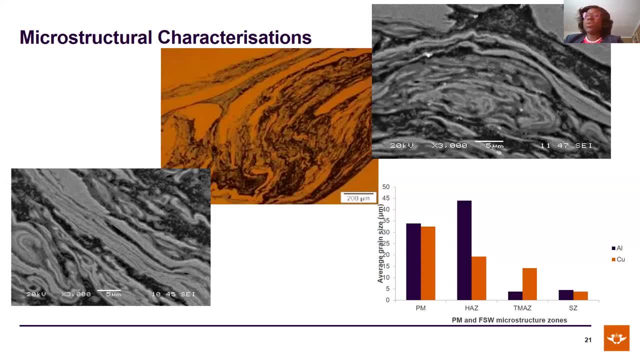 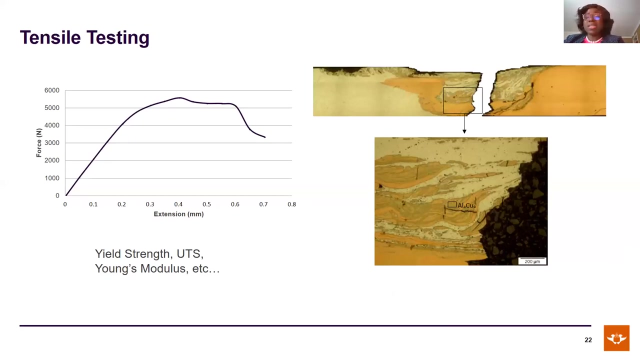 parameters have been very appropriate. So we also measure the grain sizes across various zones and we characterize them into various zones which can be directly correlated to the microstructures of various zones of the welds. We also consider tensile testing. This is a basic one wherein, as a researcher, 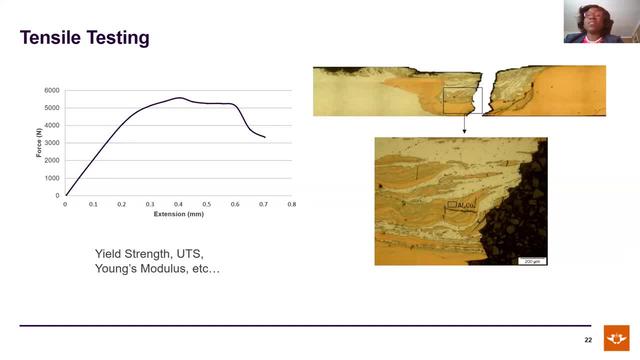 we consider the yield strength, the UTS, the Young's modulus and so many other data that we can get from tensile testing. It is also expected that researchers- researchers- should always consider fracture characterizations in the welds. Now for welds generally. this particular weld I've shown you on the right-hand side. 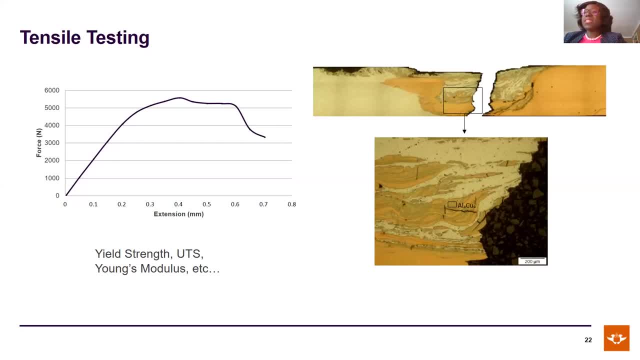 if you look at it very, very closely, you will observe that this particular weld has fractured just about the TMAZ, the thermo-mechanically affected zone. It is expected when welds are characterized can be given. terms of has been good, it is expected that the weld should fracture. 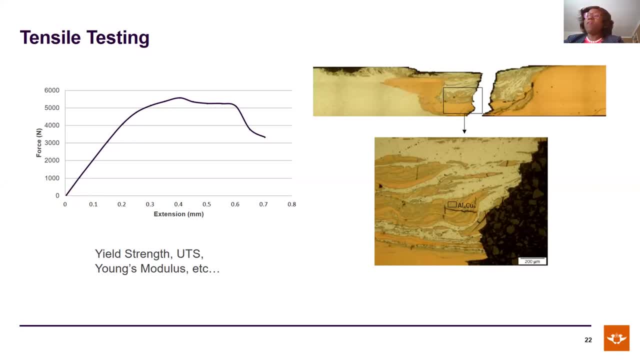 at the heat affected zone, completely outside of the steer zone and also outside the TMAZ, which is a good indication that there's a good bonding of the two materials that have been joined. This sample, this example, I've shown you here. you will see where this particular tensile sample 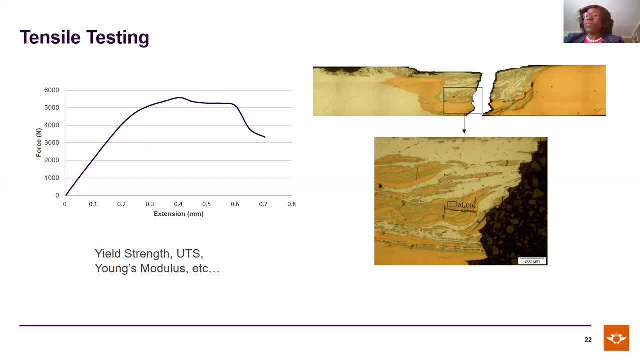 has fractured in the TMAZ, wherein these particular fractured samples were further characterized and it was found that this particular patient-steer weld welded on the TMAZ has fractured in the TMAZ and that patient-steer welded aluminum and copper has some intermetallics And 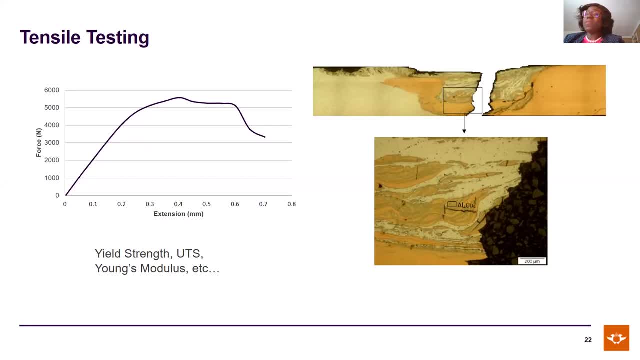 intermetallics made the weld brittle. although further details later revealed that the intermetallics in this particular, in most of the welds produced in this study- had very low peaks, however, still made the weld to be brittle. Hence they are not good for structural applications. 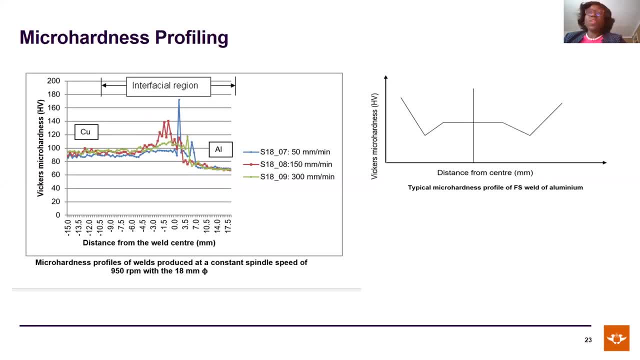 as the case may be. And now to this. Another basic characterization which we will always conduct is micro hardness profiling. The picture on the right-hand side gives typical VCAS micro hardness profiling of friction-steer welds of aluminum. So when aluminum and its alloys are welded, the steering 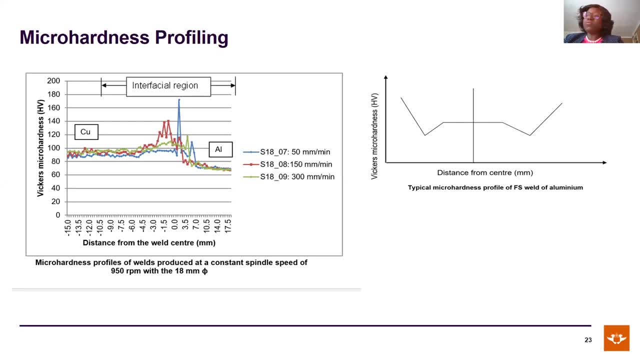 roller Fit P. write on displayでしょう. singing during the welding process usually leads to a softening And this softening then leads to have the hardness of the of of the steel zone as stable. Looking at, looking at the, the plate tool that is observed in the right-hand side corner, But if you look if you want, as you are not standing, you can ask to your classmate to cope with this, The USDM스� komma on the left. You should computing the unraveling along the easy pathwise of when Oyere pulled off these screaming tons of Well. most of all, two of the holds are strong, totally in the hanging position. shock at the left-pod, part of a close anyway. So it is, Fellan, cannot bottom shoe towards you If you hadn't handled your guards well thus that you wouldn't have been able to. 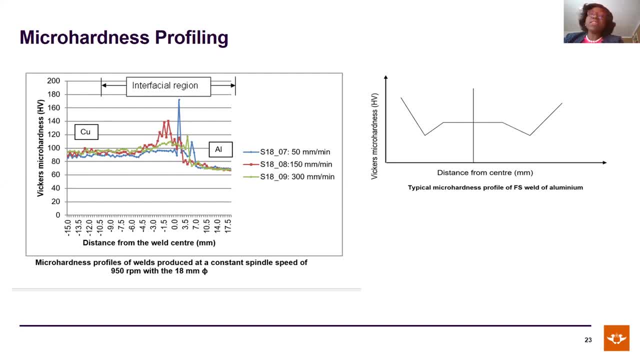 help. However, in this study, this shows exactly what you need to do. You can top up Pass jerk method. Look at the micro-hardness profiling on the left-hand side. This is for aluminum and copper. You will see some peaks at the steer zone. 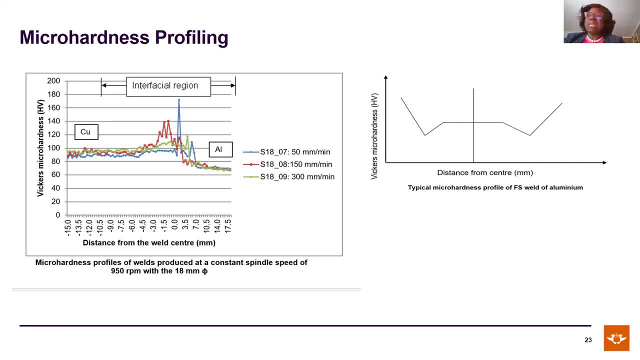 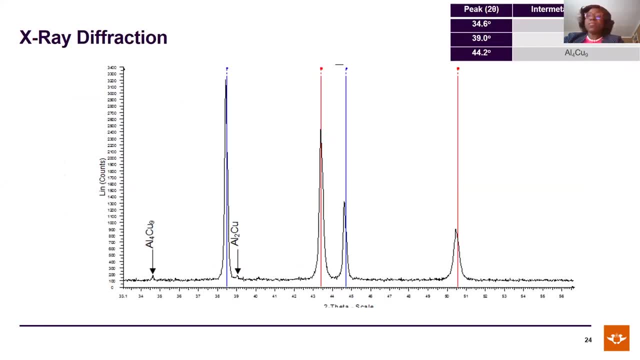 which correlates to the intermetallic compounds that are present in the welds. This is ester diffraction of the similar aluminum and copper weld. If you look at the top right-hand corner, I have placed in there the various peaks at which these common intermetallic compounds. 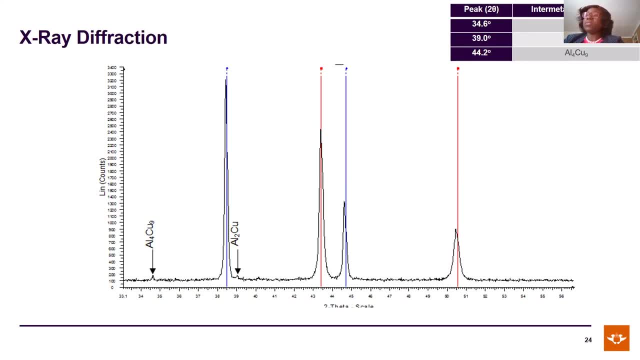 will trigger in the welds. So we have 34.6,, 39, and 44.2 for the various intermetallic compounds. Now, looking at the diffractor graph, you will observe the very low peaks of two intermetallic compounds. 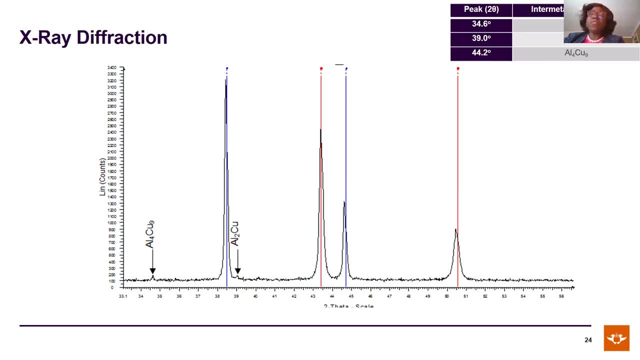 that are found in these particular welds, The aluminum and copper intermetallic compound that is found in the welds. So these further confirm to me that the welds, yes, they were intermetallic compounds, but then they are not. 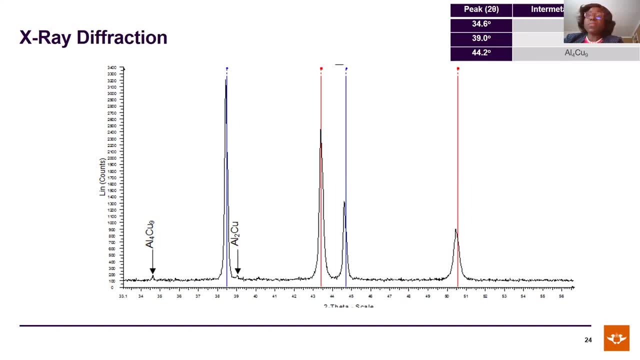 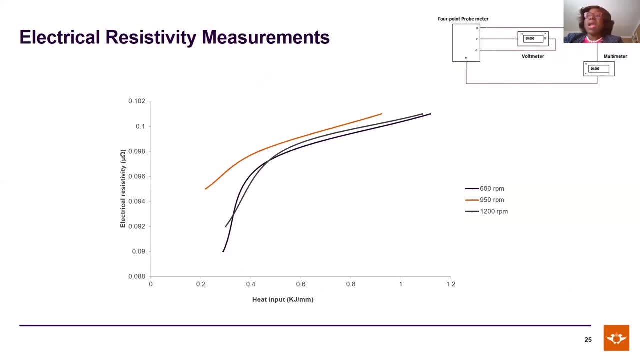 they do not have very high peaks. You can, we can- see the low peaks there that have been picked up using the X-ray diffraction And for that test, because we are looking at aluminum and copper in the electrical and electronics industry application. 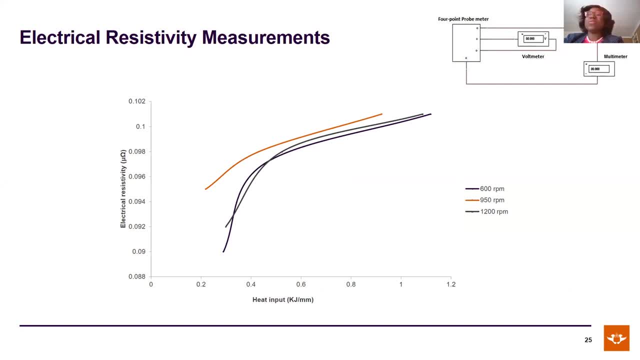 we had to conduct electrical resistivity measurements to be sure that the material the welds produced is fit for use, And this was done using the four-point probe meter. The schematic is placed on the top right-hand corner. We have the voltmeter, the power saw, the multimeter. 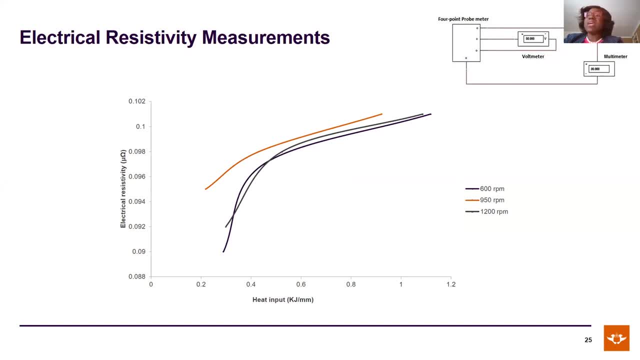 and then we place the sample with the four-point probe meter, wherein we carefully placed two probes on aluminum and two probes in the copper, with having the sample of the friction-steer welded sample. So this the results, the data obtained. this is what I have. I have this graph here. 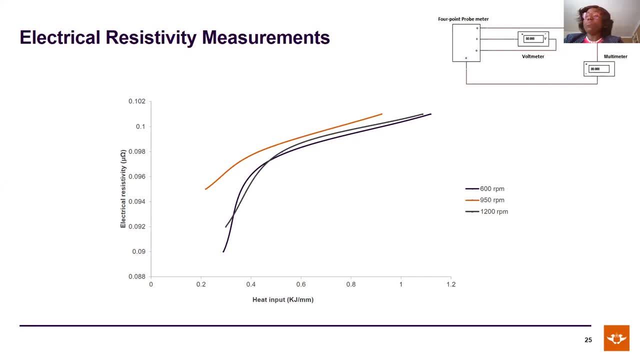 which is indicating the electrical resistivity in microohms compared to the heat input into the welds, Because the heat input is correlated. the heat input into the welds is correlated to the formation of the intermetallic compounds, in the sense that 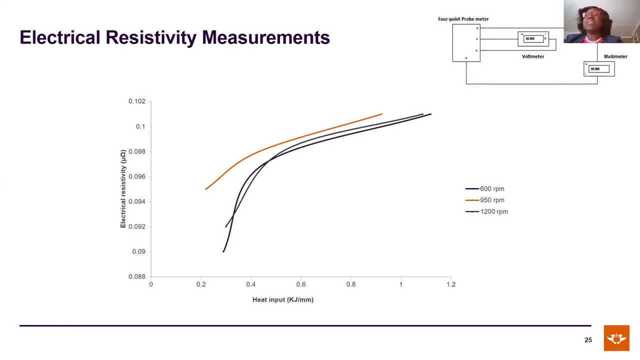 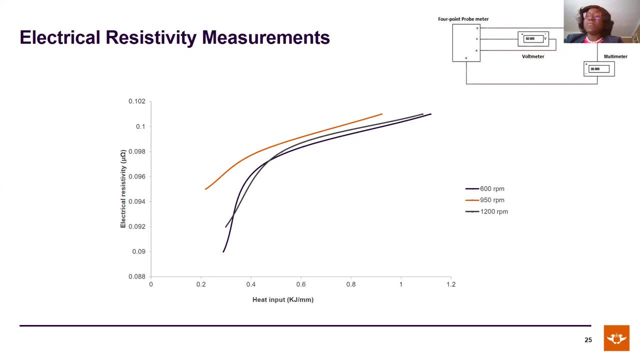 We observe. from the data that is before us this afternoon, you will observe that the electrical resistivity are very, very low in microohms, and that is the data we have here. So with this we were able to to optimize the Frisch & Steyr weather samples of aluminum and copper. 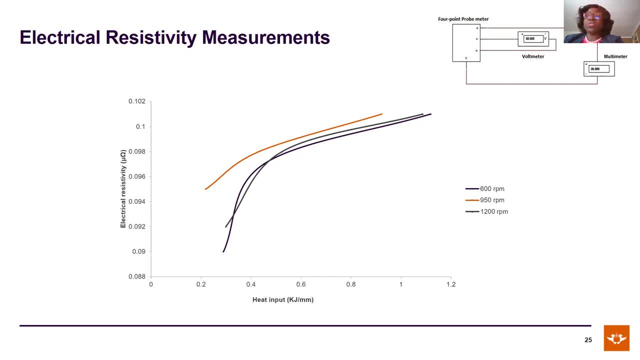 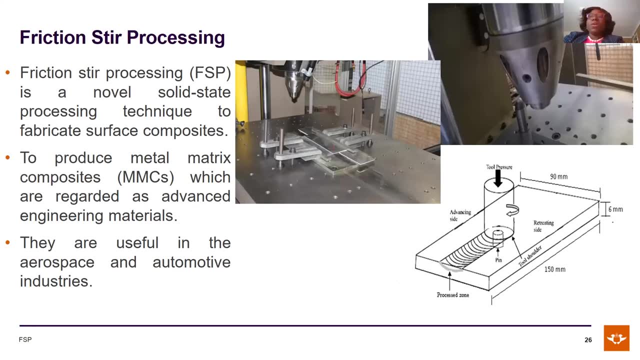 and this was used in the electrical industry in both bars. So I would like to the next one or two slides will speak to. I will highlight some work that we have done in the field of Frisch & Steyr processing And this is a variant. 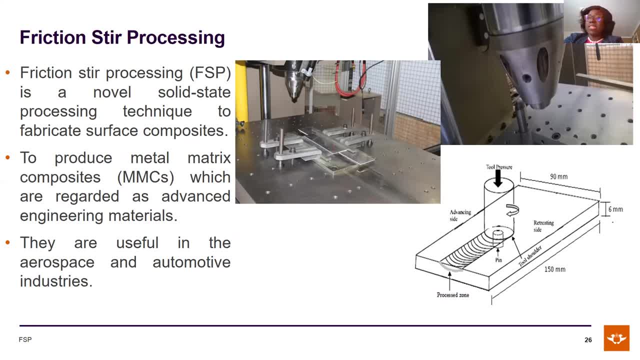 the FSP is a variant of the Frisch & Steyr welding technology. It is also a solid state processing technique that is used to fabricate a surface composite, as in surface engineering, in trying to in trying to modify the surface morphology of materials. 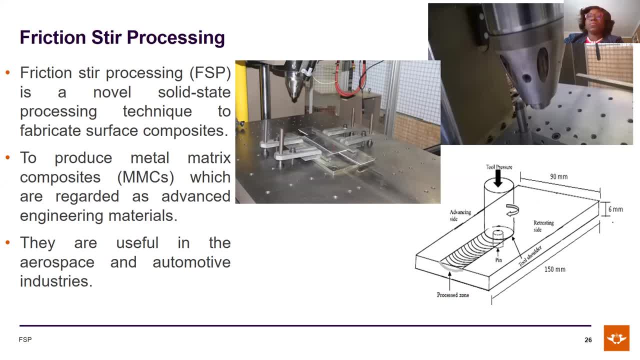 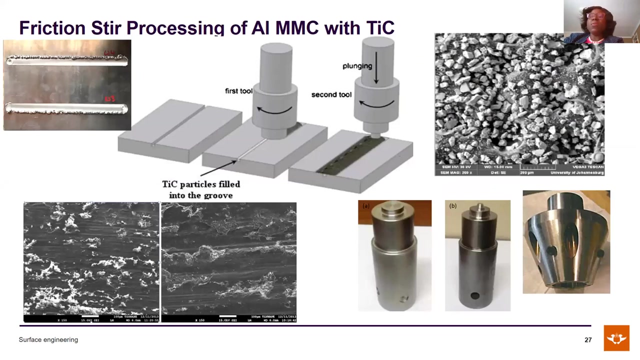 that has some limitations. The technology has also been used widely to produce metal matrix composites, and these materials have been regarded as advanced engineering materials and they find applications in the aerospace industries and in the automotive industry. The way this, the way we produce our FSP, is that we 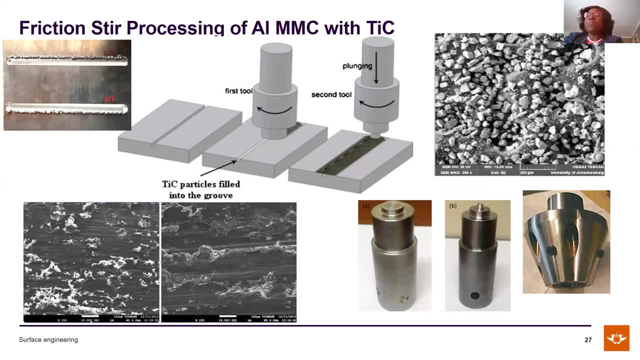 we have a. we manufacture groups in the substrate, the parent material to be used. We have grooves in them and then we pour harder materials that we want to use to reinforce the surface morphology in the groove. In this particular study, 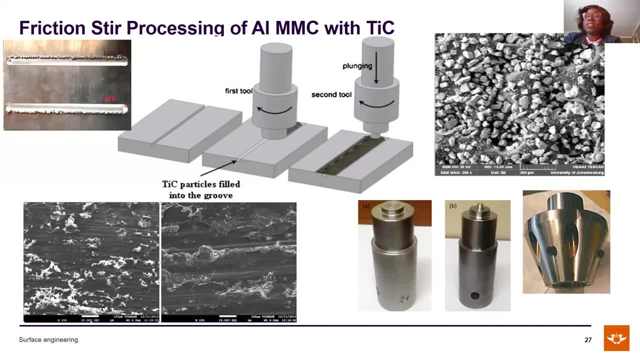 is one of my students that did this study, which I supervised. we used titanium carbide powder, particle size of between 45 and 90 microns, we poured into the groove and we've then first of all, used a tool without shoulder. 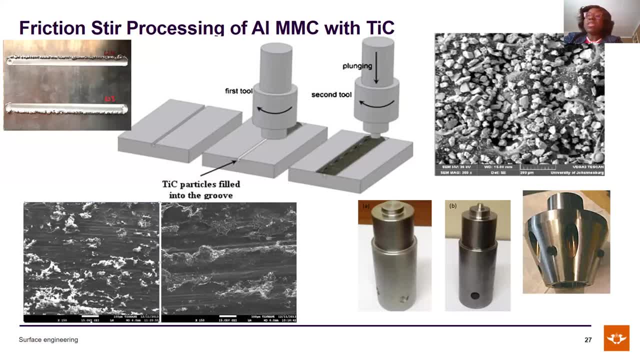 to consolidate the particles into the groove. That is what you have there as stage number two, And we use the tool on the right hand side corner of my slide tool designated as A without a tool pin. We first of all use that tool. 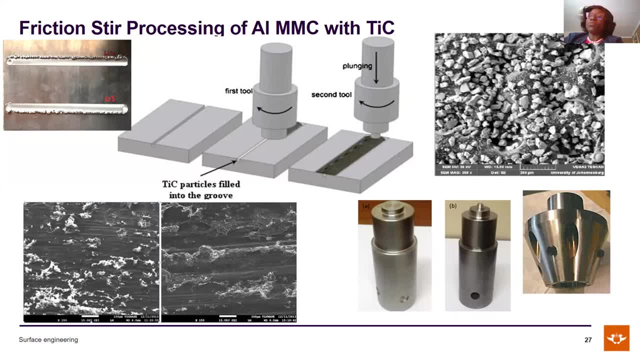 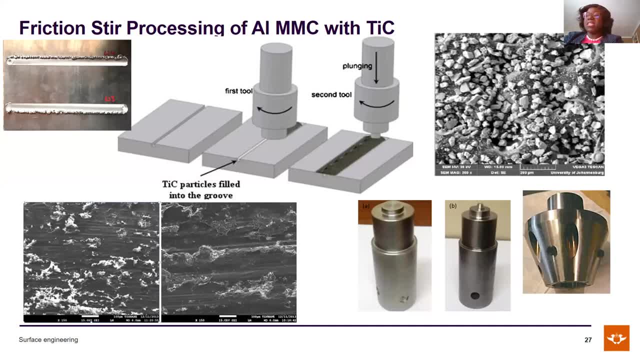 which is tool designated as B in this. in this case, we then use the tool with a pin to to to perform the friction stair processing, And this particular study was aimed at improving the wear properties of aluminum alloy. We observed that, because of the ceramic nature of TIC. 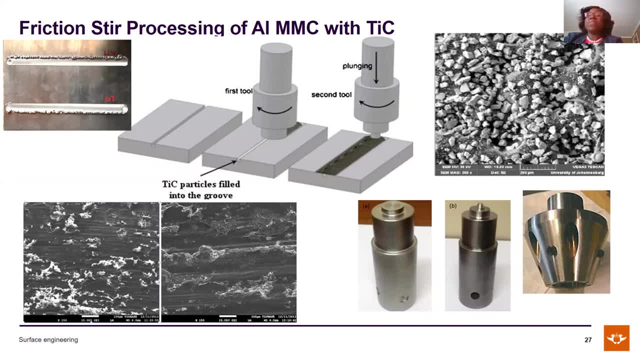 these greatly improved the properties, the wear properties, of the aluminum material in in question in this particular study. So several other material characterizations were also conducted as as well. But our most priority in this particular study is the wear study. This is where I've shown you the two wear tracks. 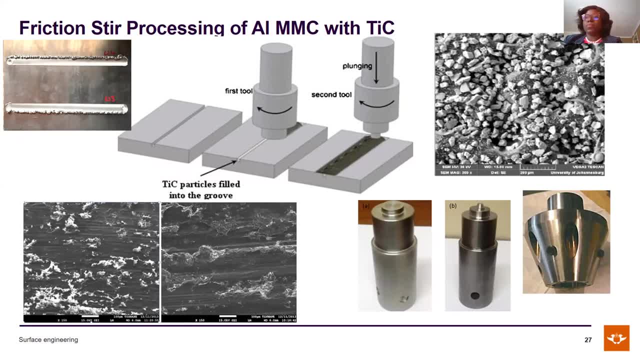 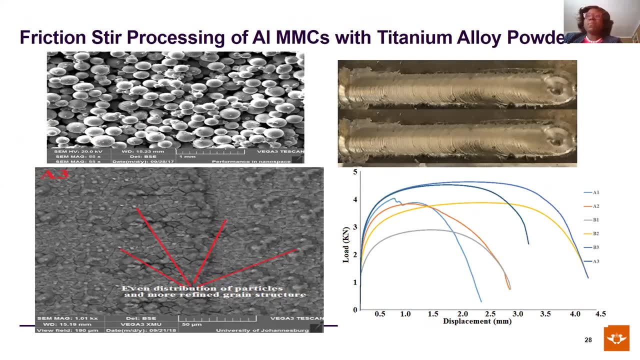 that we got from this particular study In another study, also producing aluminum metameter composite, this time around with a titanium alloy. we follow the same process as well to have titanium alloy with five to enhance the, the, the, the strength. 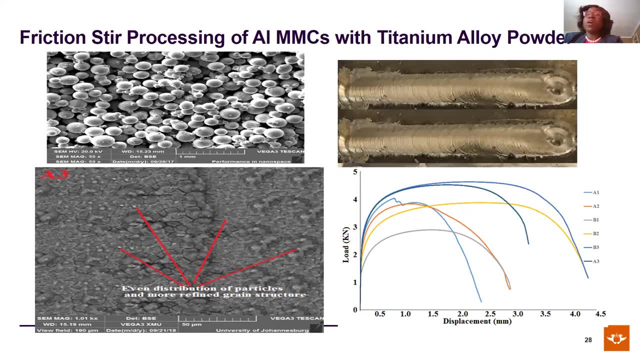 strength to weight, strength to weight to weight property of of the aluminum material, And these improved greatly the strength of the, of the mat, of the of the material that was produced. You will see the microstructure taken with with the same. 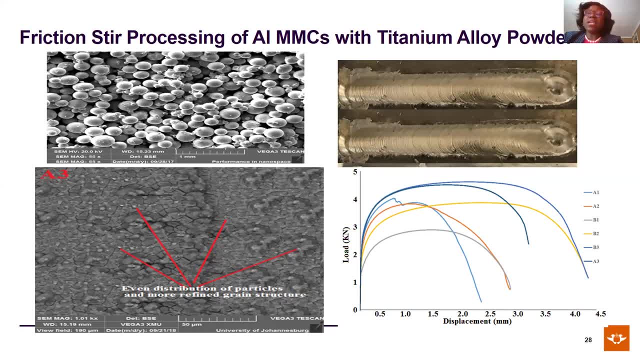 how it's showing that an even distribution of particles and very refined grain structure of the aluminum and titanium particles at the steer zone of the friction steer processed aluminum metameter composite. This study was also very successful- was published and we're also considering some applications as well. 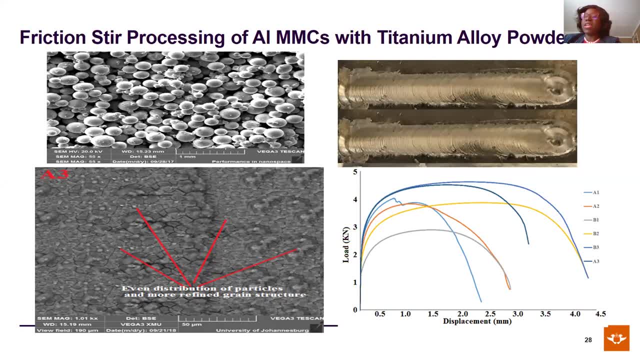 for this particular study. I've also shown here, on the bottom right-hand side corner of my slide, some of the of the tensile results showing the, the ductile behavior of the of the of the friction steer process, the aluminum MMC. 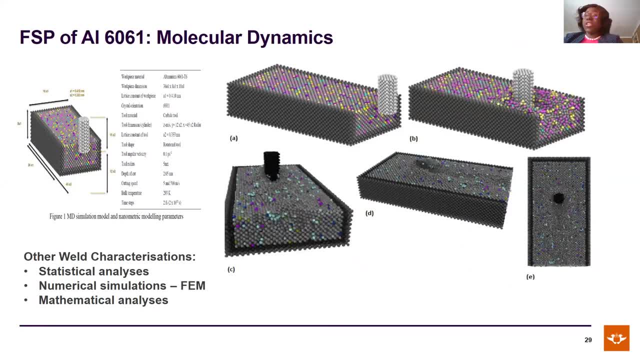 Okay, Now still on materials characterization generally. there are so many other materials characterization techniques that are that have been developed and have also been been been used, and many are still being developed. So a student of mine also did some work wherein we used molecular dynamics. 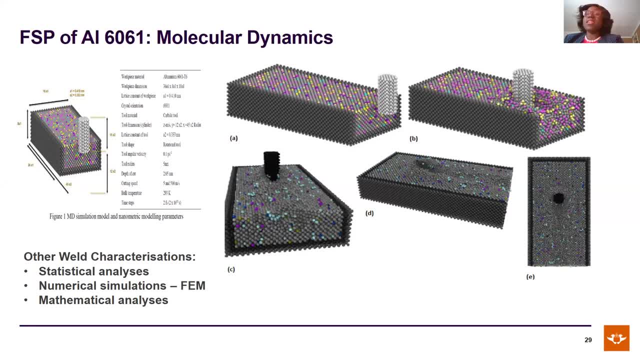 applied it to to to quantify the strength, the outcome of friction steer processing of aluminum 6061.. So these are some of the these are some of the outcomes of of that study. Now other world characterizations that are also widely used by researchers is to consider. 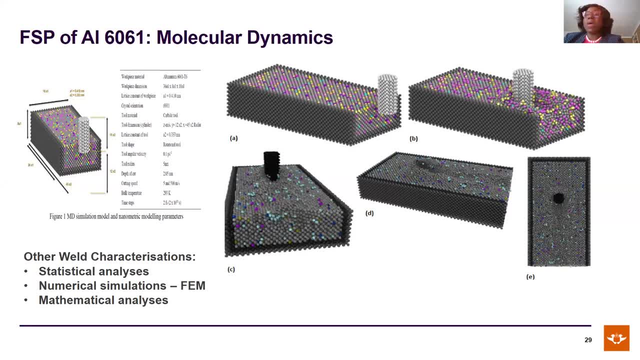 statistical analysis, various software design experts and so many other software that are available in the open literature that can be used to characterize worlds. There are also so many numerical simulations using FEM, many softwares that have also been used to characterize worlds. 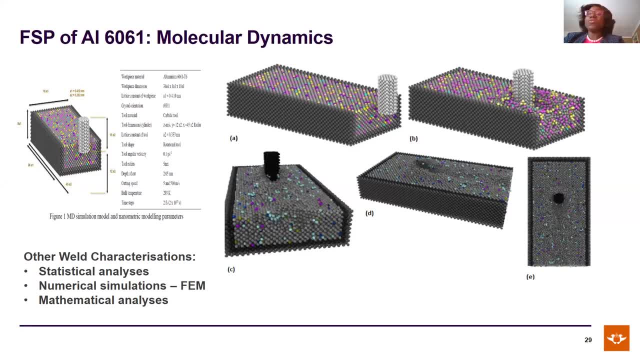 And also there are opportunities for a lot of researchers also go into mathematical analysis And for for me and my research team, we have been, I would say, 85 to 90% experimental, within a little bit of, yeah, experimental and statistical analysis. 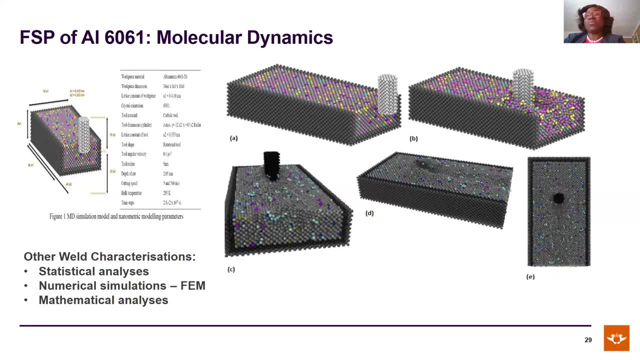 That is. that's the core of what we do in my research team. A lot of our, a majority of our work we do, we, we, we, we, we conduct materials characterizations through experiments and we also conduct statistical analysis as well. 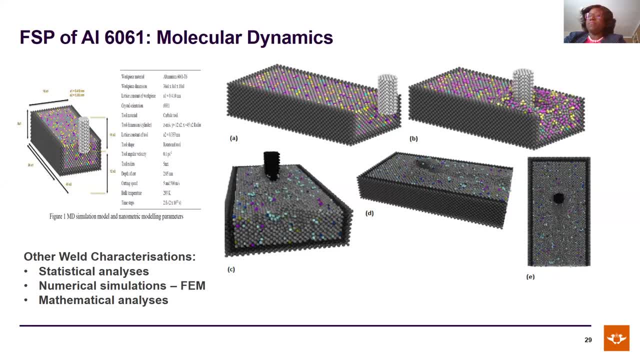 And then a few students have delved into numerical simulations using software, like this one student that used molecular dynamics. I've also had one student as well who used the ANSYS and a couple of other work as well, But still at developmental stage. 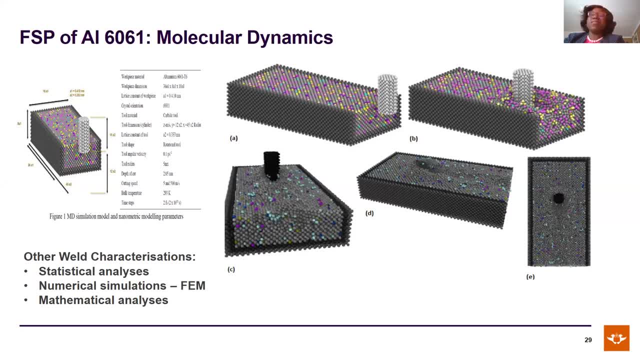 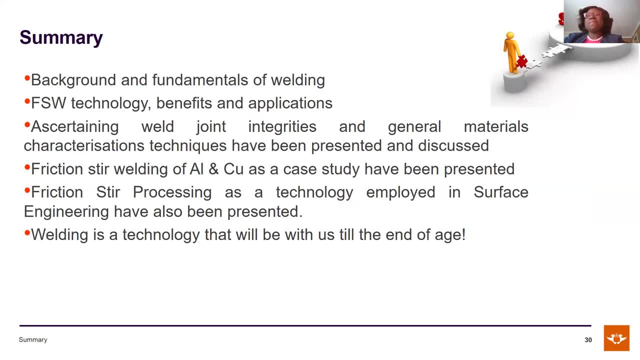 I would not consider myself as an expert in the in numerical simulations and mathematical analysis. So, having said that, I'm coming towards the end of my of my talk. To summarize, I have shared with you this afternoon background and fundamentals of welding generally. 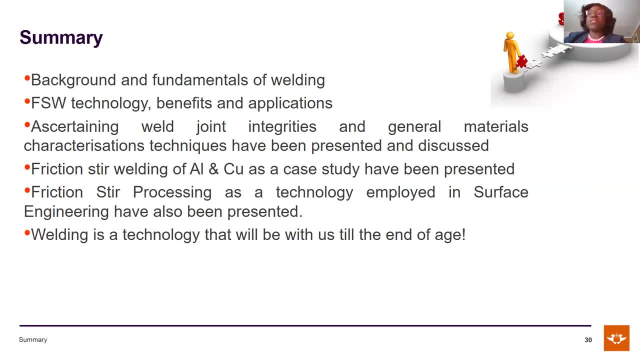 In particular, I have shared with you my experience in the field of special steel welding technology, various benefits, its applications, commercial applications, also at a research and development level as well. I've also shared with you how, as researchers, 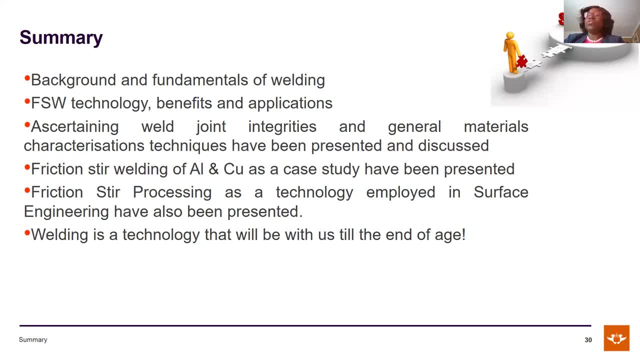 we need to ensure that we ascertain weld joint integrities and also general material characterization techniques that we should consider in, in, in in carrying out weld characterizations. I've shared with you a typical case study of special steel welding of aluminum and copper. 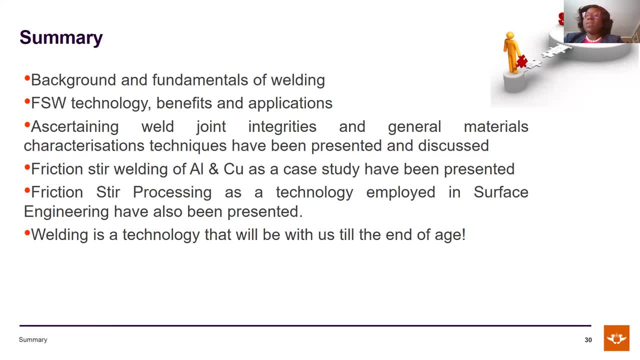 Shared with you special steel processing as a technology, how we have used it in surface engineering to produce aluminum metameter composites And, with this background, I believe that you will all agree with me that welding is a technology that will be with us. 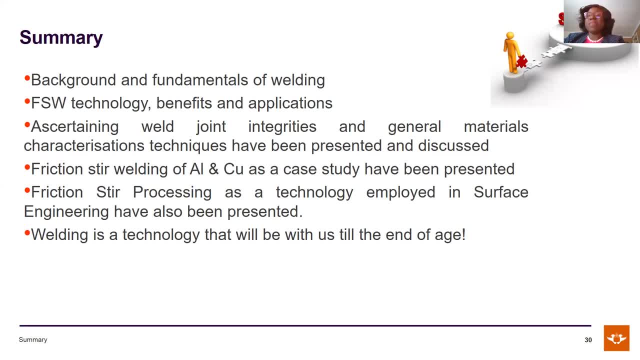 till the end of the age. So as this, this particular field of of, of, of, of technology, this particular technology, will be with us for quite a long time, because we always need to join two materials together. Very 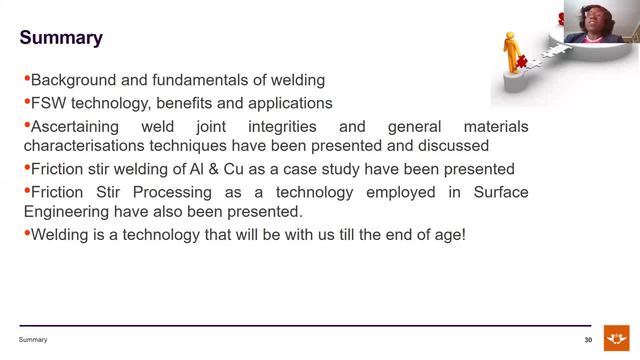 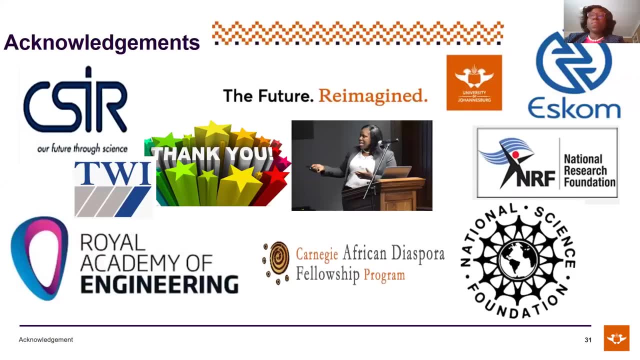 very important And hence the field of researchers. the number of researchers in the field of welding generally continues to grow every day. On that I would like to acknowledge my funders uh, the Center for Scientific and Industrial Research in South Africa. 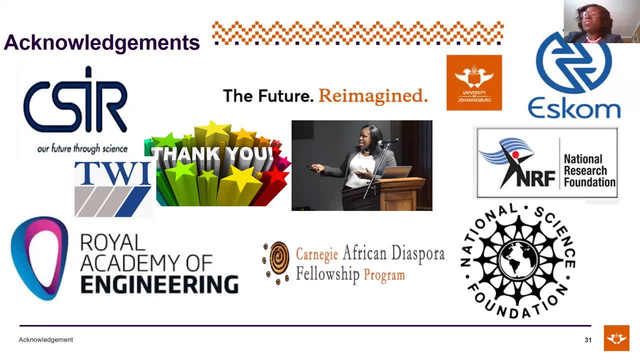 the Royal Academy of Engineering, the TWI, the University of Johannesburg. I've received some fellows from the Carnegie African Diaspora. I've had some funding, you know, funding from the National Research Foundation in South Africa. Also some funding from the National Science Foundation in the. 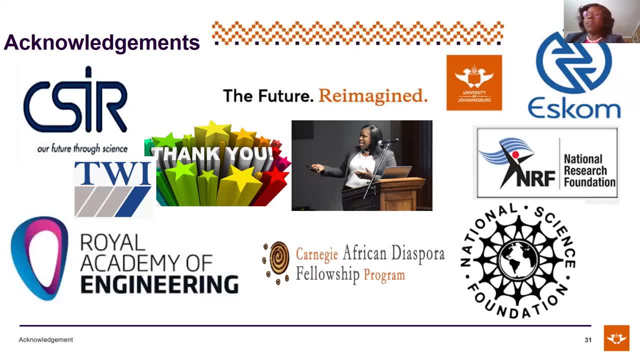 in the US, uh from ESCOM as well, and a couple of other funding bodies that have contributed to my research in the last uh 11 years that I've been. I've been uh working as a faculty member. 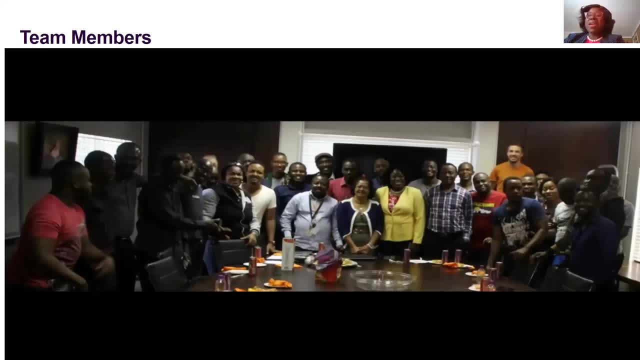 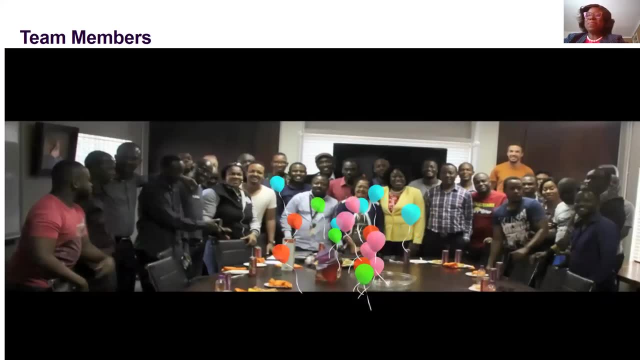 I would also like, anytime I make presentations, I like to always uh acknowledge my wonderful team members. I mean very large research uh group at the University of Johannesburg. uh many masters, PhD and doctoral studies. 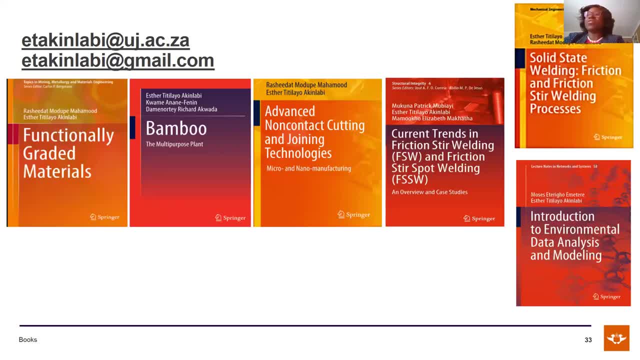 that, uh, that work in the research team to uh for that And, uh, this particular slide I have been able to. I've been privileged to co-author six books in the field of uh, fission steel welding. 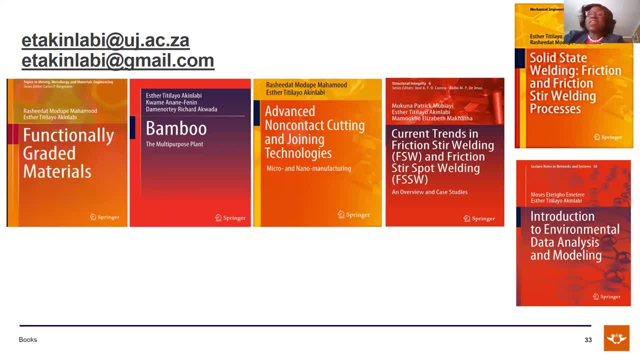 in the field of uh laser additive manufacturing, functionally graded materials, bamboo, and also non-contact welding and joining technologies, and all of that. All these books are available on Amazon if you are interested in any of them, if you.